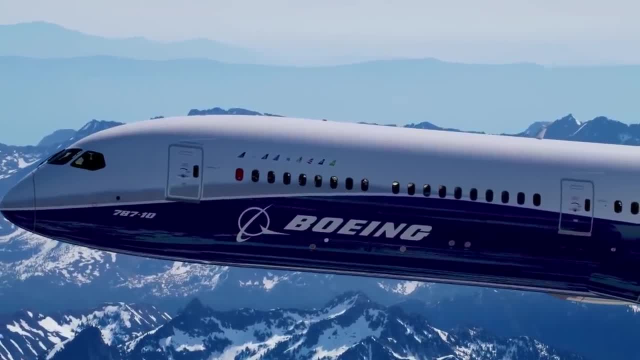 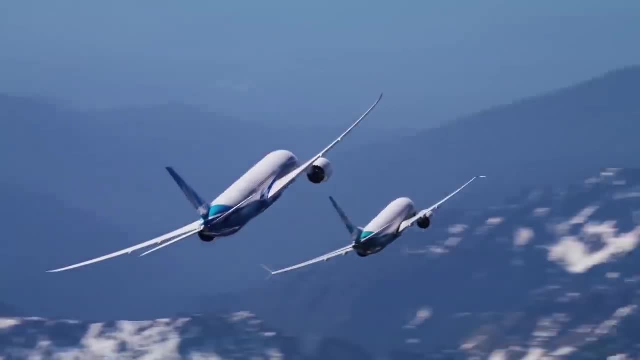 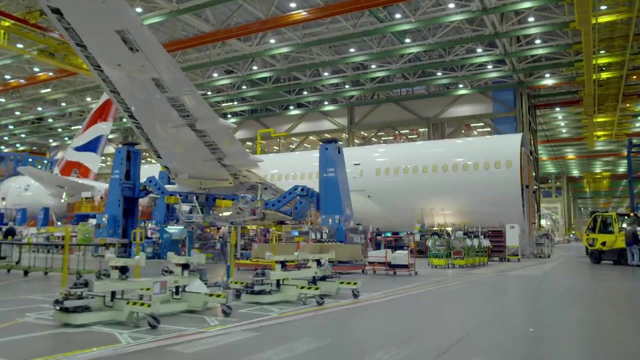 Boeing sat at the poker table and pushed all their chips forward. An all-in bet on a radical new future, and it paid off. The 787 revolutionised not only how the airline industry operates, but how the future of planes will be designed and built. 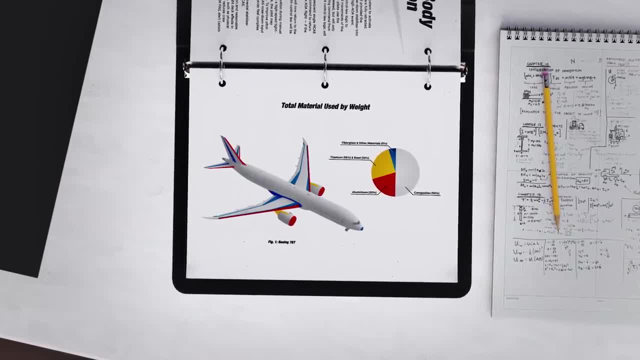 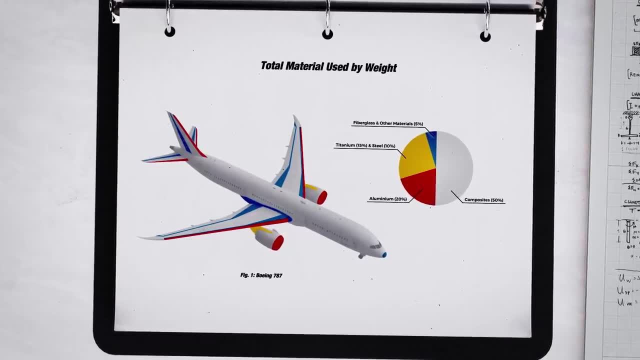 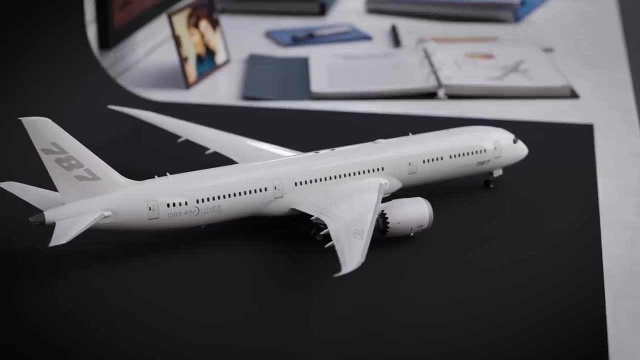 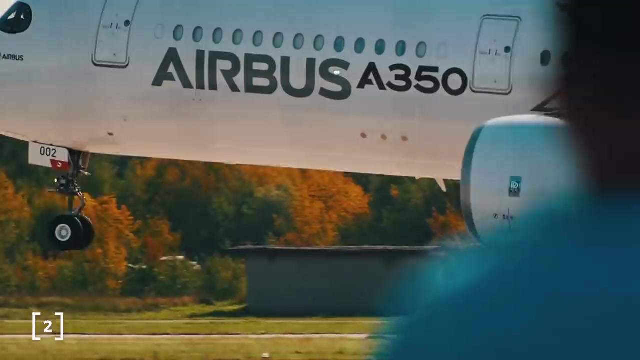 This is the breakdown of the 787's materials By weight. 55% of the 787 is made from composite materials like carbon fibre reinforced plastics, making it the first commercial airliner made primarily with this new age material. The 787 is rivalled only by the Airbus A350 XWB, introduced 4 years after the 787, in 2015.. 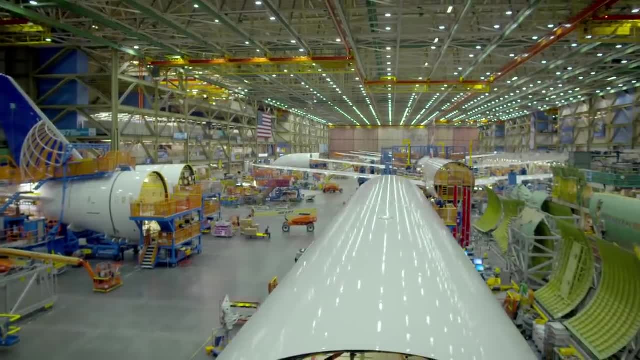 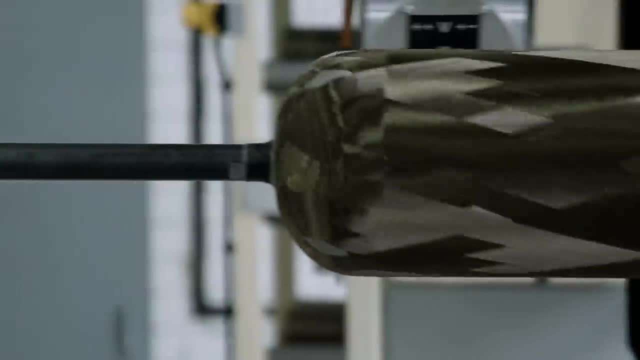 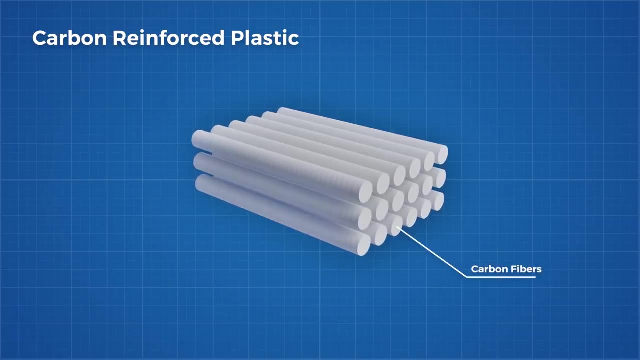 So why are composite materials so desirable for the airline industry and how has the 787 made the most of their advantages? Composite materials are made up of two or more materials. Like carbon reinforced plastics, they are composed of extremely strong carbon fibres bound together by a plastic resin. 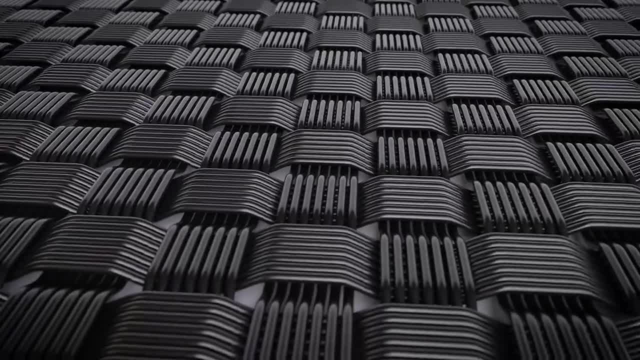 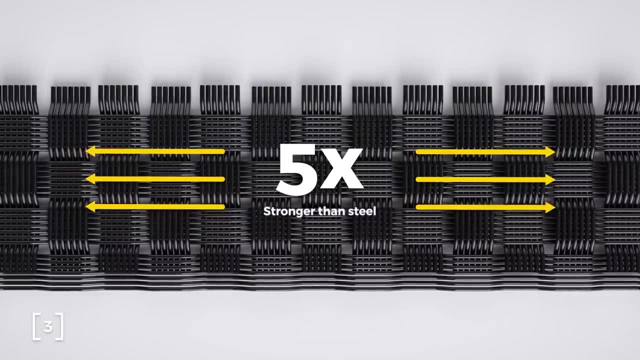 Carbon fibre, made up of thousands of tiny, thin fibres of carbon, is incredibly strong in tension, up to 5 times stronger than steel and 1 fifth of its weight. But these tiny fibres can't create a solid part by themselves. 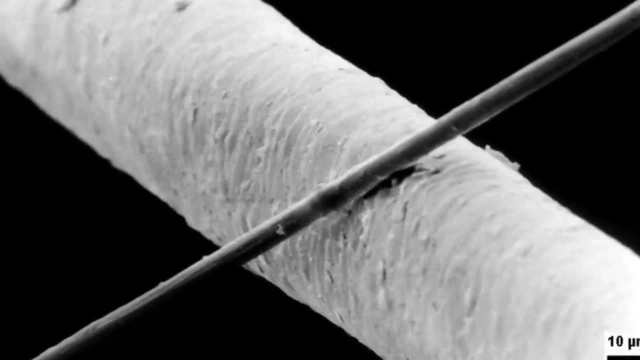 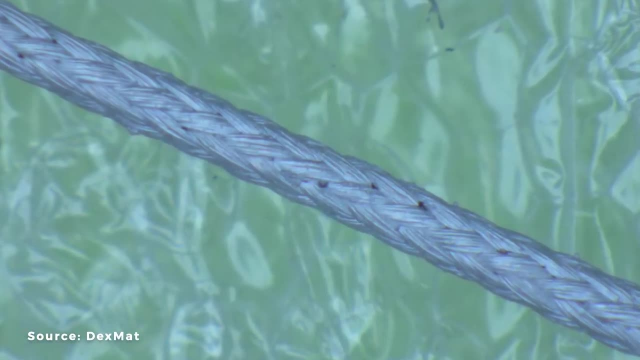 This is an image of a human hair beside a carbon fibre. This is an image of a human hair beside a carbon fibre. This is an image of a human hair beside a carbon fibre. The carbon fibre is the smaller one And, just like a human hair, they can bend and flex and separate very easily. 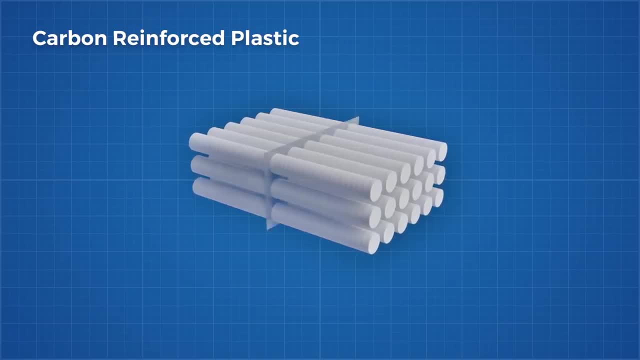 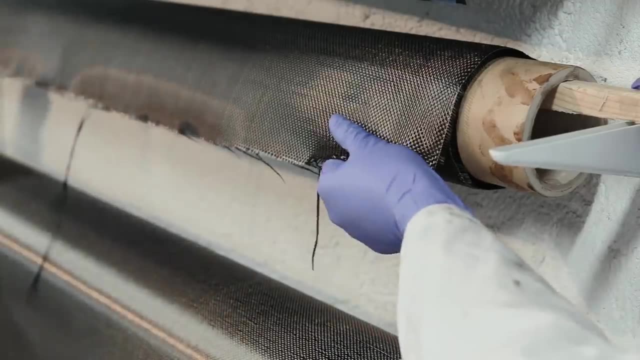 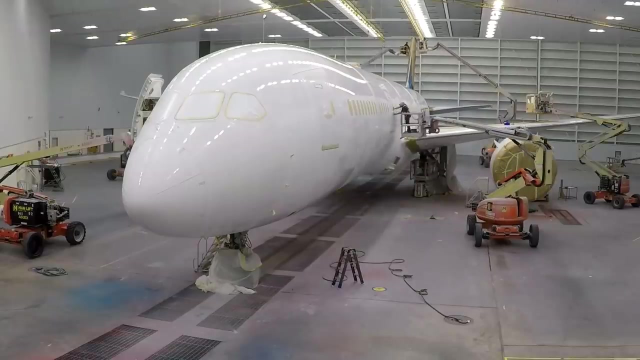 So we need to first bind them together with a plastic resin to form a solid material. Otherwise they just form a strong but flexible fabric. That flexibility as a fabric is exactly what makes composites so useful when creating the precise and elegant curves of a plane. 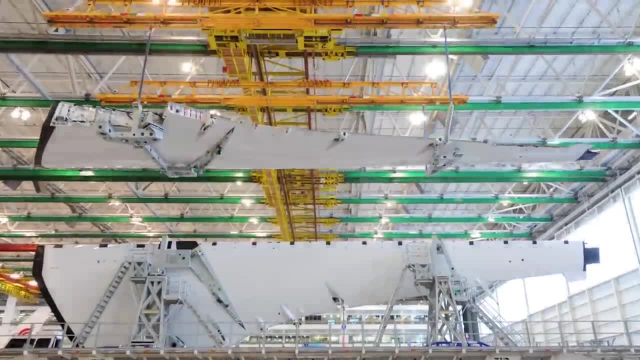 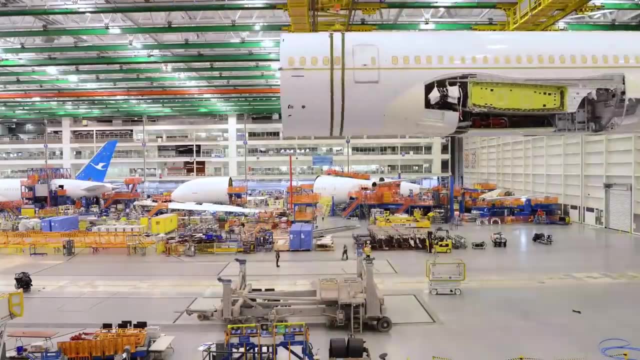 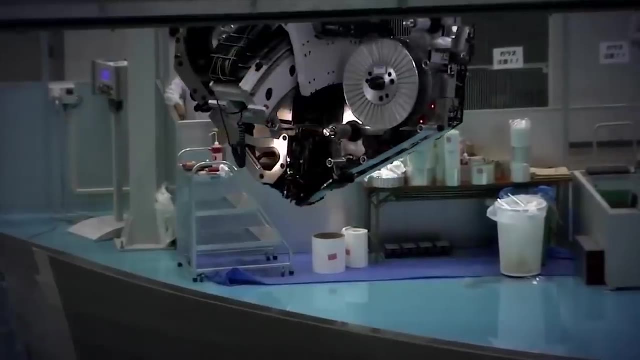 With the right tooling and designers, Composite components can be made into almost any shape imaginable. In the past, a disadvantage of making large aircraft components from composites was the time taken to manually lay up parts Where layers of carbon fibre and plastic resin had to be carefully constructed. 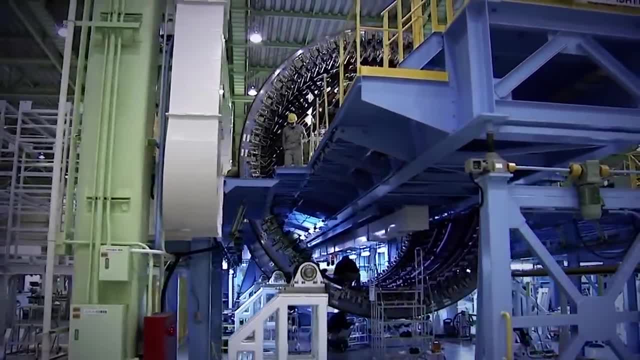 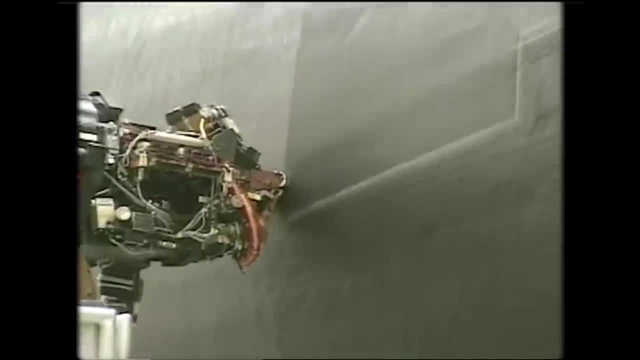 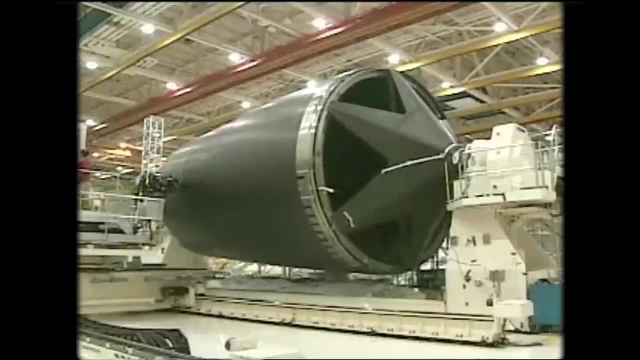 It required skilled technicians and was inherently difficult to scale to the production quantities Boeing needed. To get around this, Boeing uses automated tape laying to produce massive components. The 787's fuselage is created by wrapping a carbon fibre tape impregnated with a plastic. 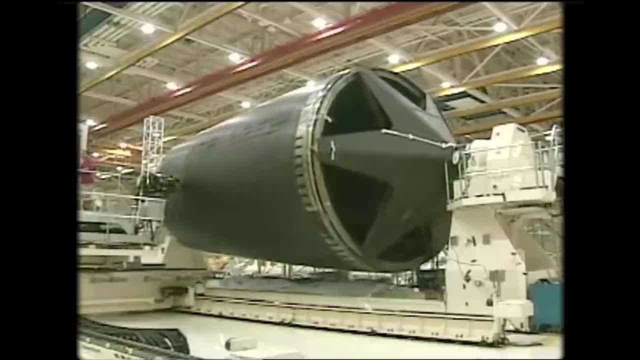 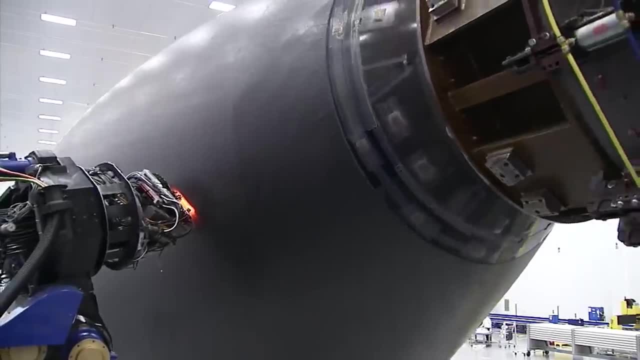 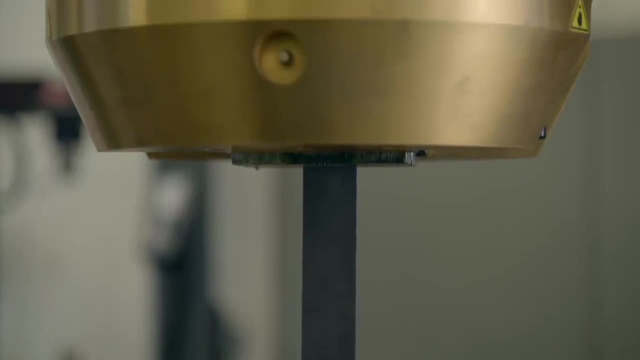 resin around a rotating mould of the fuselage. This machine precisely controls the overlaps of the tape and the orientation of the fibres to ensure we are getting the most out of the carbon's tensile strength to resist the internal pressure loads and the longitudinal bending loads the fuselage will experience. 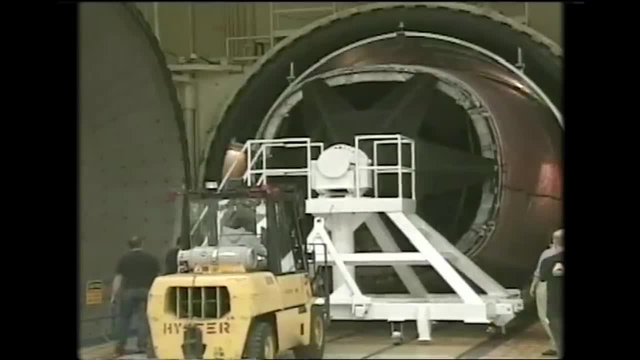 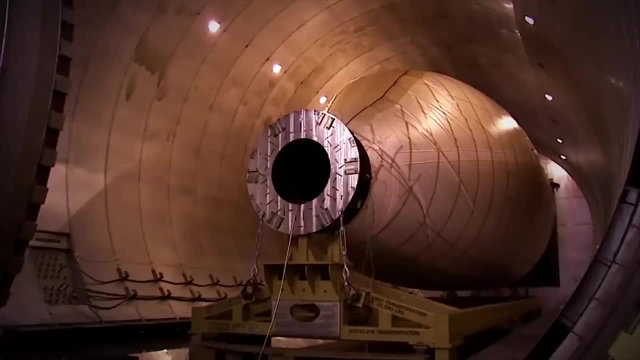 One of the problems with this manufacturing method is that the part needs to be placed inside an oven to cure the resin. This hardens the plastic and creates a solid composite structure. Ovens the size of a wide body jet airliner fuselage are not exactly common, and this 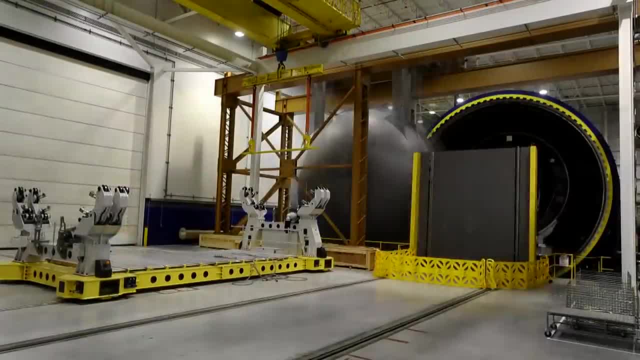 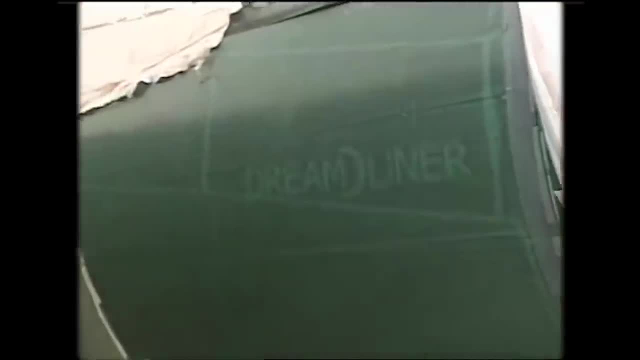 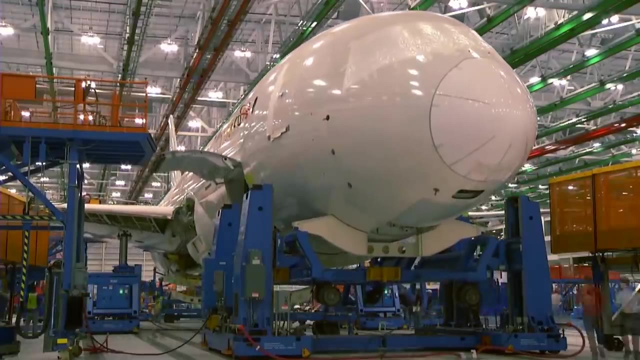 is often the limiting factor on parts made this way and requires massive upfront investment to build a customised oven large enough to fit the part. but the benefits are well worth it. The first and most obvious is the strength carbon fibre provides. Previous generation airliners are typically pressurised to an equivalent of 8000 feet. 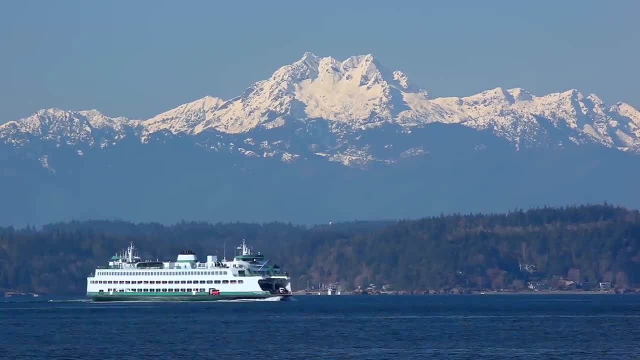 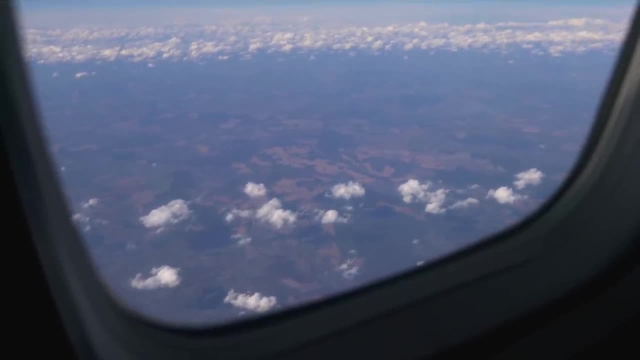 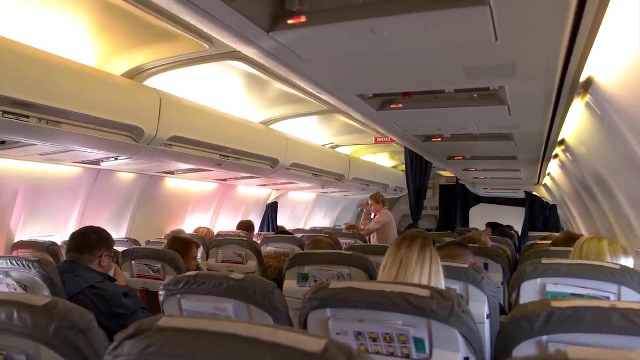 that's the same height as Mount Olympus in Washington state. High enough that the lower pressure would reduce your oxygen intake and your stomach will bloat, as the air inside is higher pressure than the outside. This is uncomfortable and exacerbates the effects of jet lag, but thanks to the 787's, 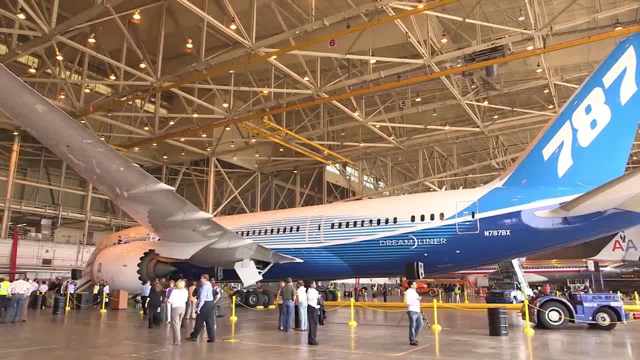 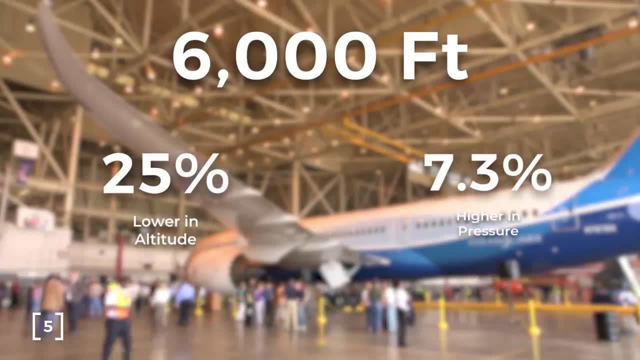 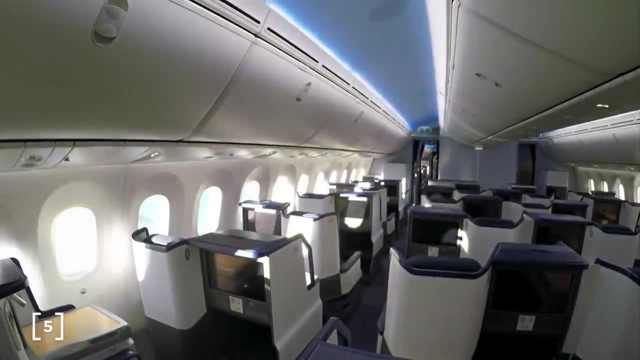 stronger fuselage, it can increase its internal air pressure to an equivalent of 6000 feet, 25% lower in altitude and about 7.3% higher in pressure. That may not sound like a lot, but it goes a long way in making the journey more comfortable. 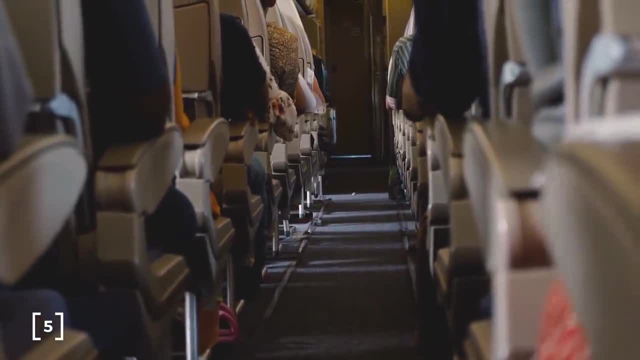 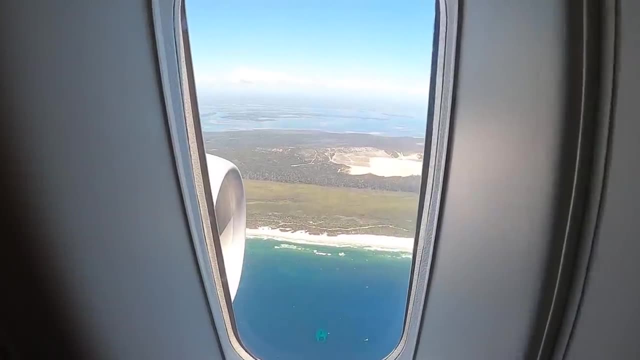 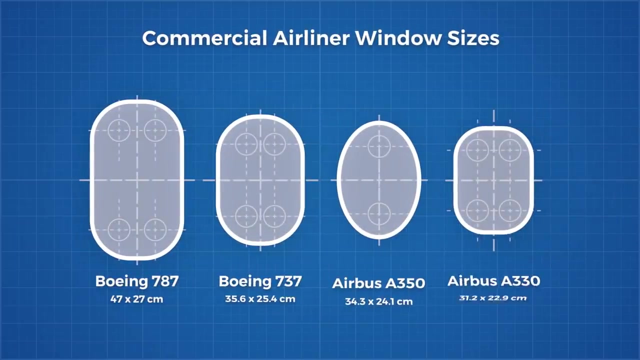 And, at the very least, the person next to you won't be farting as much. Less farting is always nice, but my favourite benefit of the stronger fuselage is the absolutely massive window. This is the 787 window, and these are windows of some equivalent aluminium airliners. 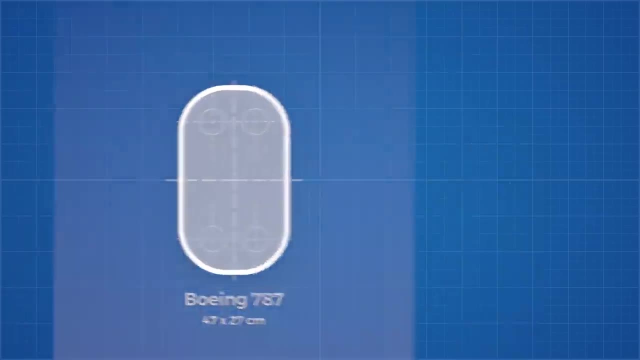 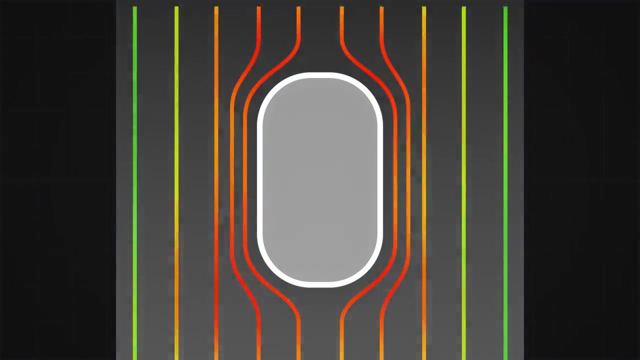 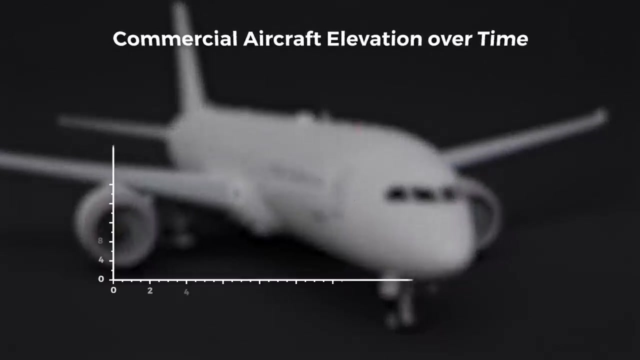 They are absolutely massive In aircraft made primarily from aluminium. having holes this large in metal panels would result in the build up of stress at the window boundaries. as the stress contours have to deviate around the window, This stress does not exceed the material strength. but over repeated pressure cycles, tiny imperfections. 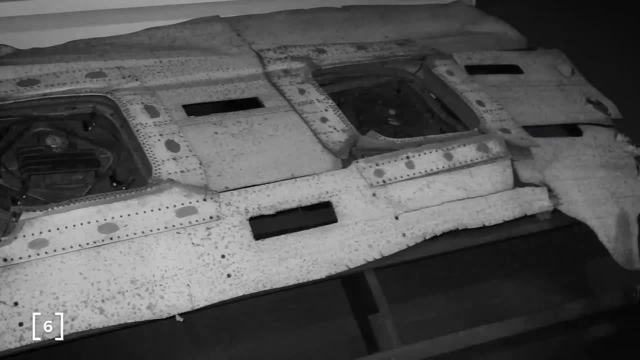 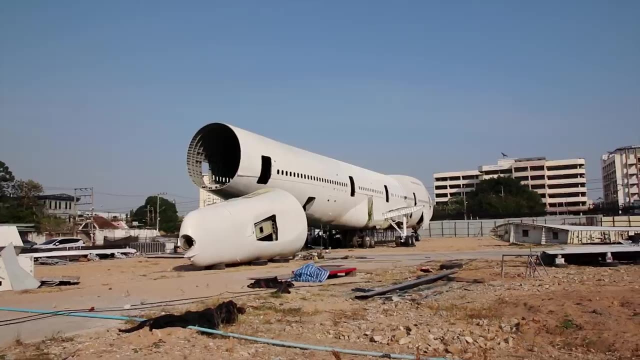 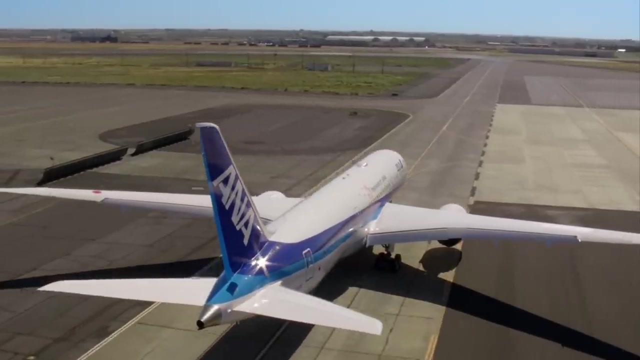 in the metal can grow into even larger cracks and eventually fail. Holes this large in an aluminium airliner would severely shorten the plane's flying career before it needed to be fixed or disposed of, Kind of like how cracks in McGregor's leg shortened his career, but it's not a problem. 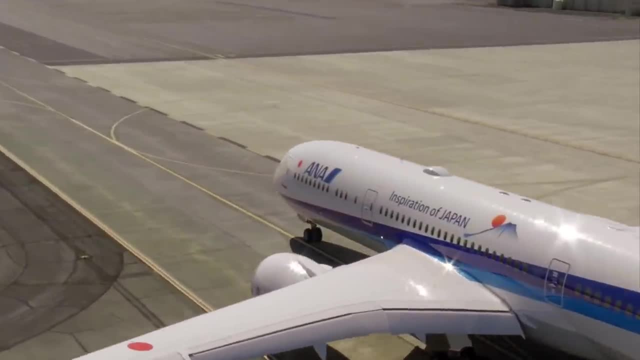 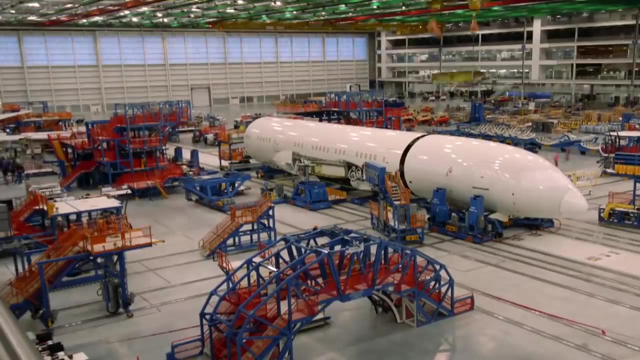 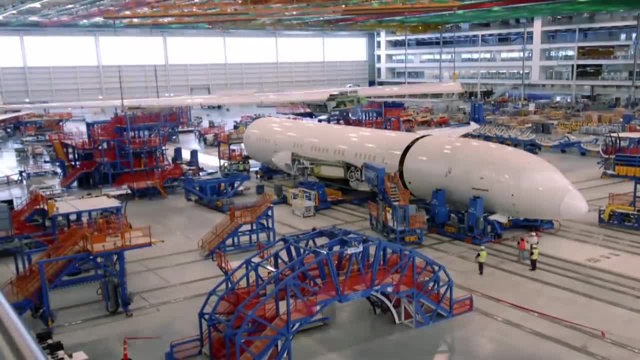 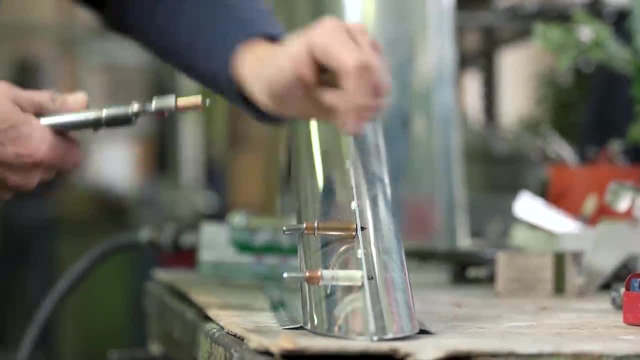 The 787 is the most powerful aircraft in the world. It has plenty of benefits for the airline operators too, because the fuselage is just one massive part. Boeing was able to eliminate all joints and all the fasteners needed to join them together. 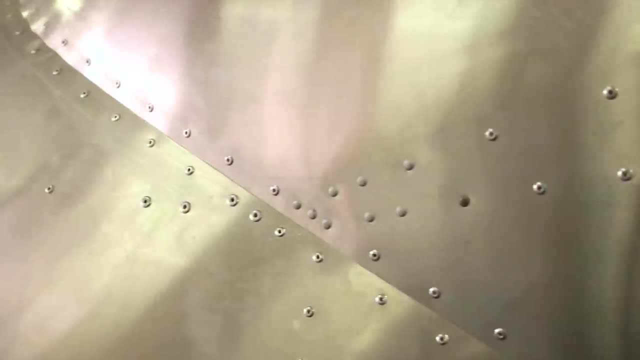 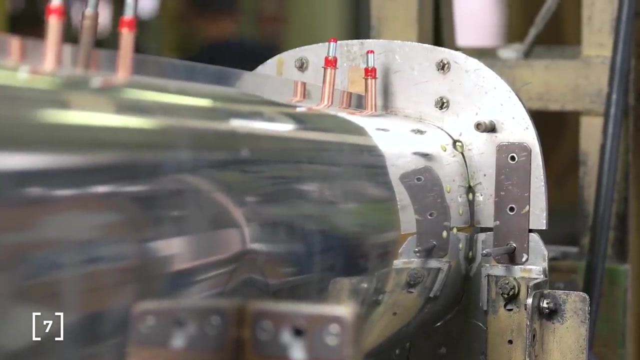 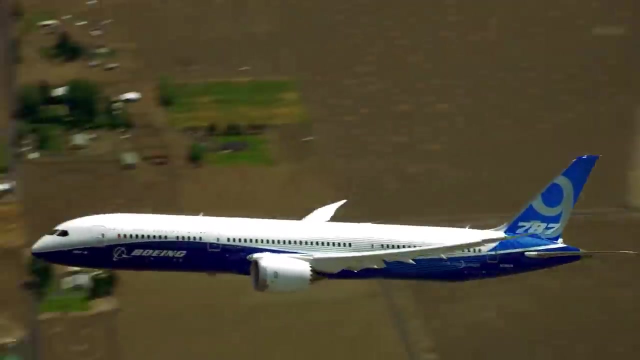 The sections that used to be made up of 1500 aluminium sheets riveted together using 40-50 thousand fasteners are now just one massive carbon fibre section. Carbon fibre's strength to weight ratio already makes the fuselage lighter, but eliminating joints and fasteners makes it even lighter again. The reduced weight reduces fuel burn. 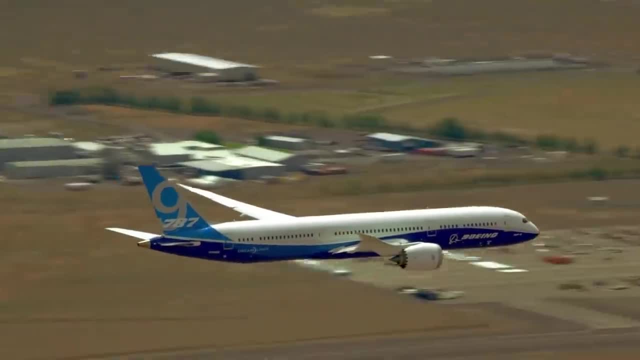 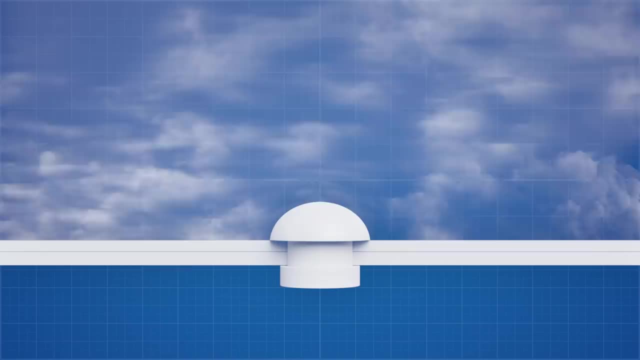 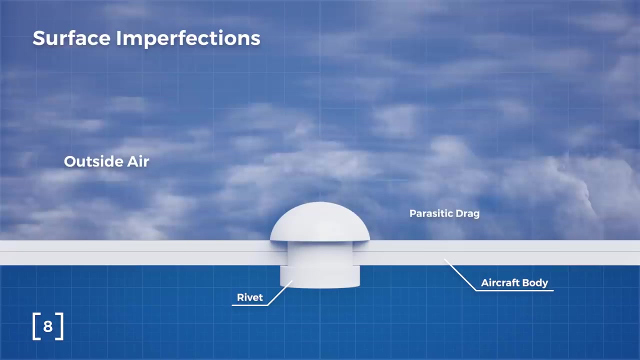 but this fuselage is also incredibly aerodynamic because it doesn't have thousands of little bumps and ridges all over it from those joints and rivets. These surface imperfections make the plane's surface rough and cause it to disturb more airflow, increasing parasitic. 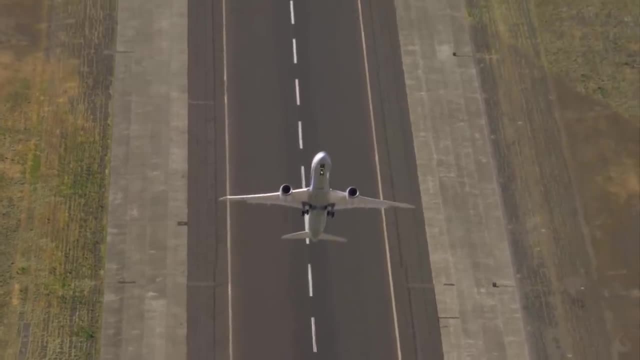 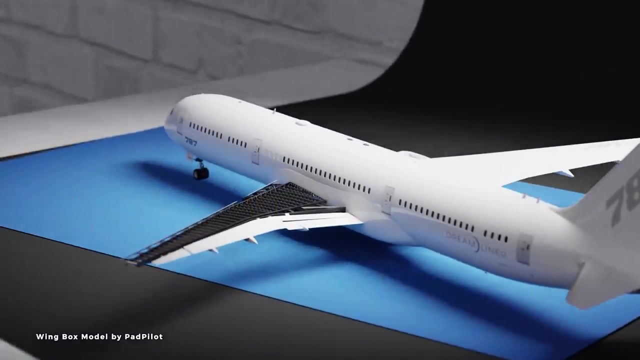 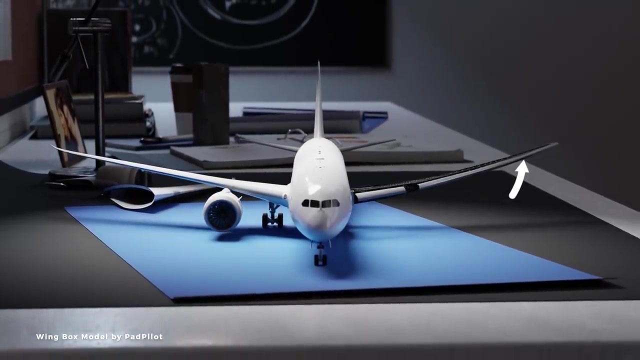 drag. Composite materials help reduce drag in other ways too. One of my favourite things about the 787 is its elegant wings. The main structural member of a wing is the wing spar. It's primary role is to resist the upwards bending force during flight. It's essentially 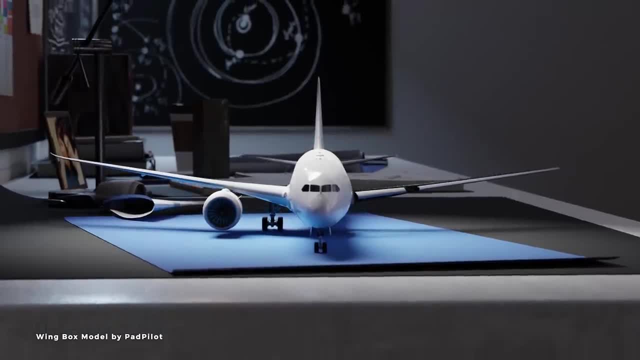 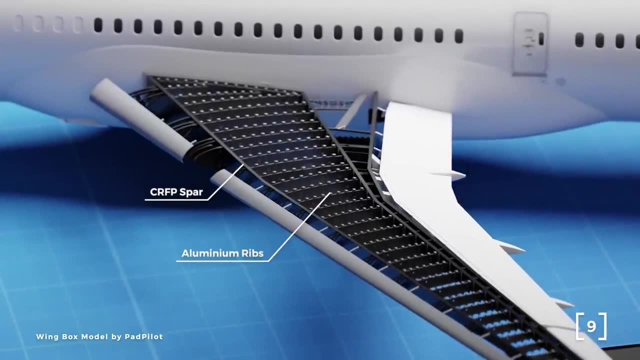 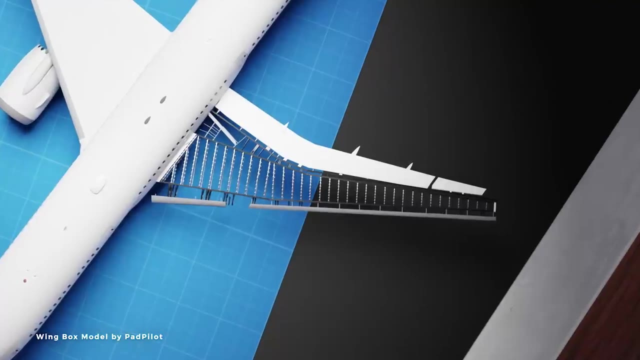 just an I-beam, a shape optimised to resist bending loads. The wing spars of the 787 are constructed from carbon fibre composites, while the ribs, the structural members connecting the two spars and that support the wing skin, are machined out of solid aluminium plates. 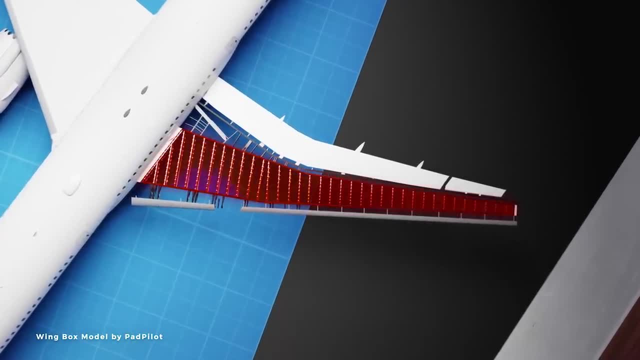 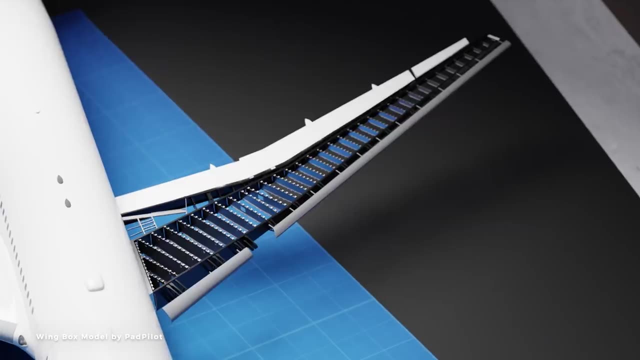 These structure, the wings and the wing spars, are made from carbon fibre composites, and the structure the rear and forward wing spars form with ribs running between is called the wing box, and it forms the main load bearing structure of the wing, while also being a 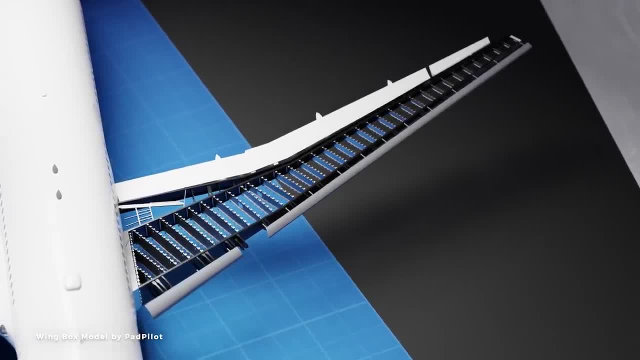 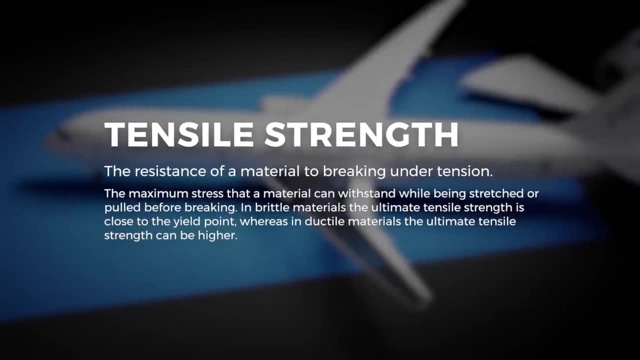 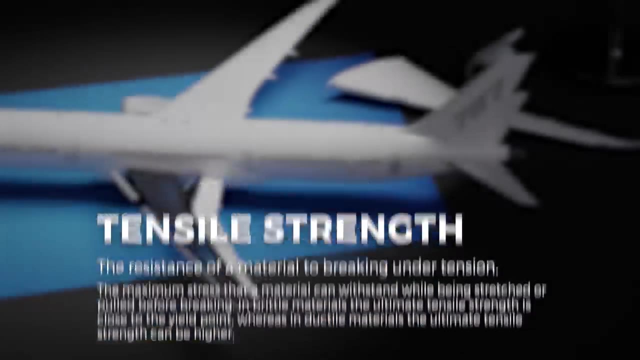 literal box for fuel to sit inside. The carbon fibre composite spar provides the wing fantastic strength. Strength is quantified by the force required to completely fracture a material. but carbon fibre composites have another important quality that makes them perfect for aircraft wings: Their maximum. 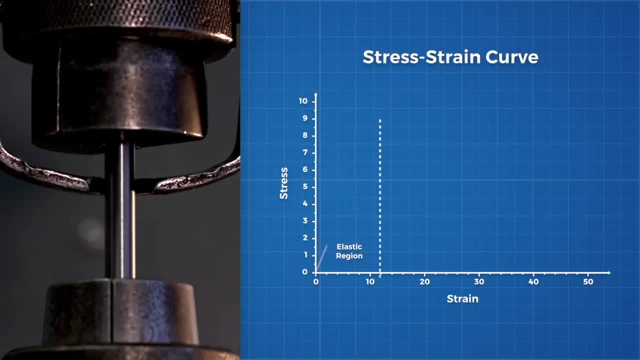 strength is their elastic strain. There are two types of deformation: elastic and plastic deformation. Elastic means the material will snap back into its original shape after the load is removed, like an elastic band. Plastic means it will permanently deform and won't return to its original shape once. 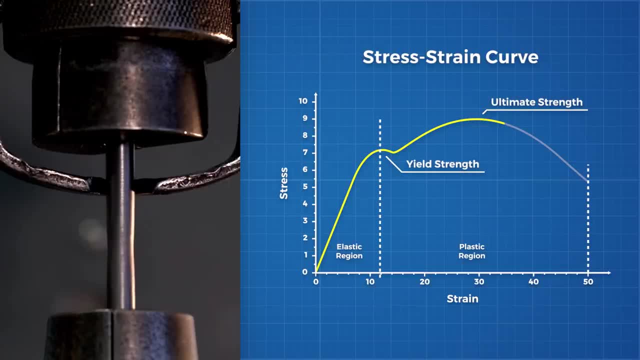 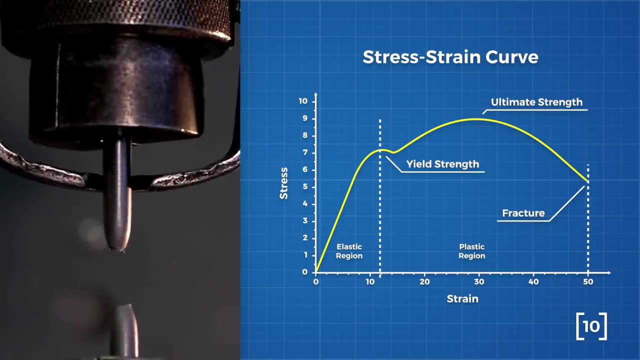 the load is removed, something we don't want to happen. This is permanent damage. Carbon fibre composites can deform further before they strike this plastic deformation- This is called the plastic deformation zone- at about 1.9%, while aircraft aluminium begins. 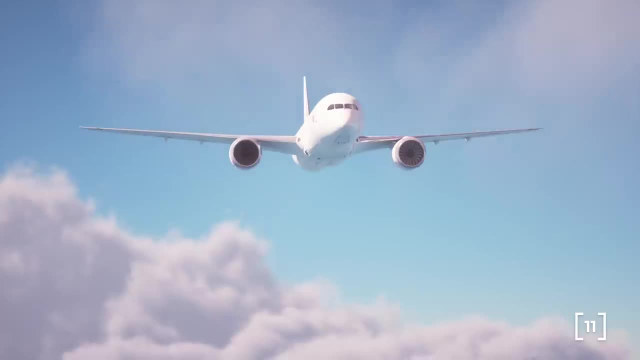 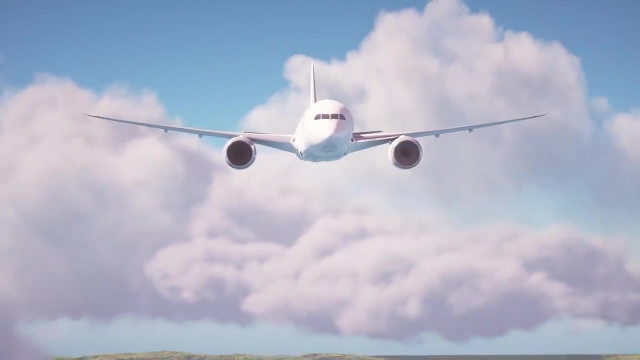 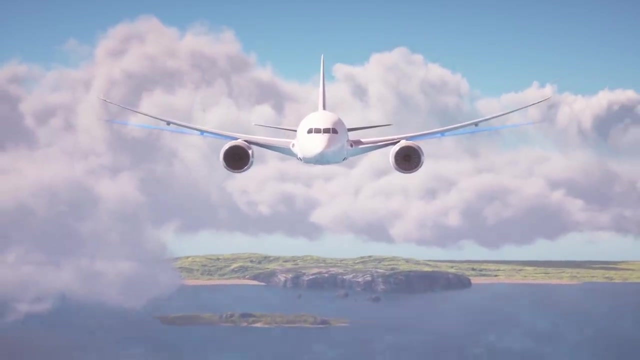 permanently deforming at less than 1%. That means we can bend carbon composites further before we need to worry about permanently deforming them, and that means we can make our wings super flexible During flight. the wing tip of the 787 can move upwards by 3 metres. That sounds like a lot, but in order. 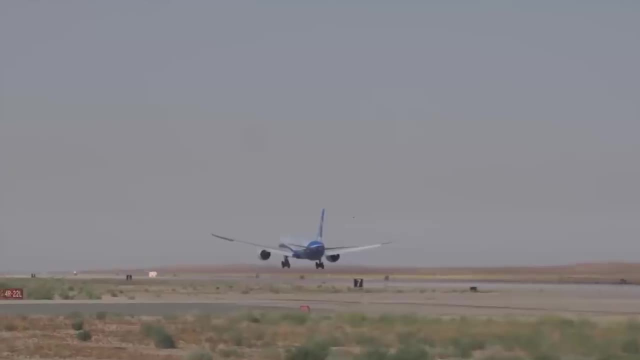 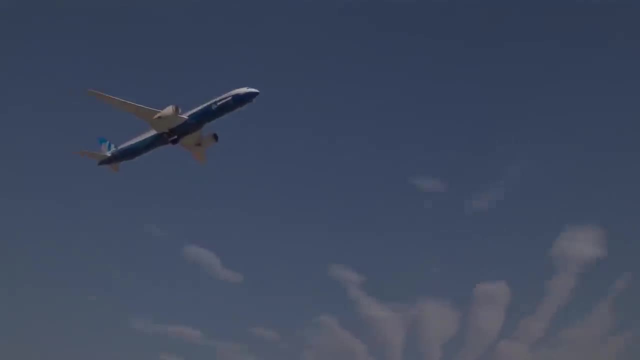 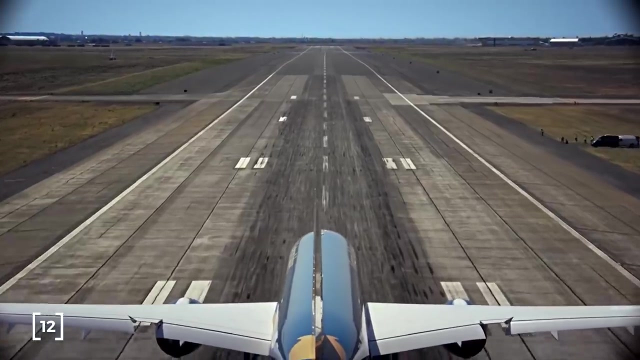 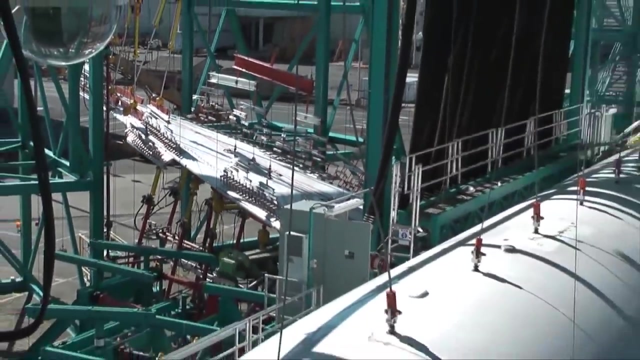 able to handle 150% of the plane's absolute maximum expected load during flight for 3 seconds, And during that test the 787's wing bent upwards by 7.6 metres. That's a great deal of bending, despite carbon fibre composites being stiffer than aluminium, meaning. 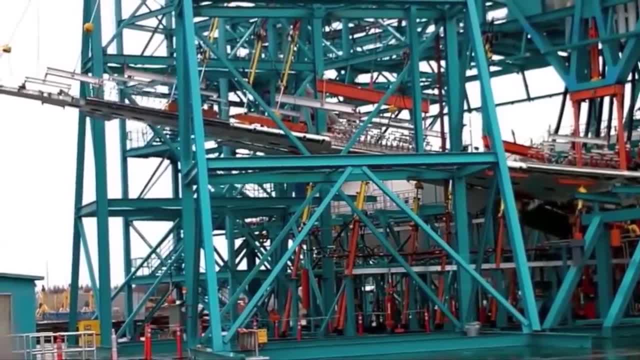 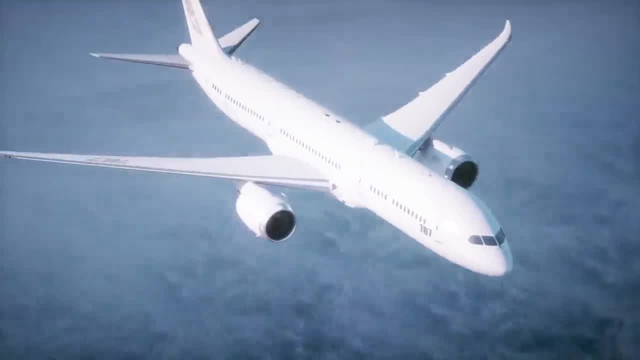 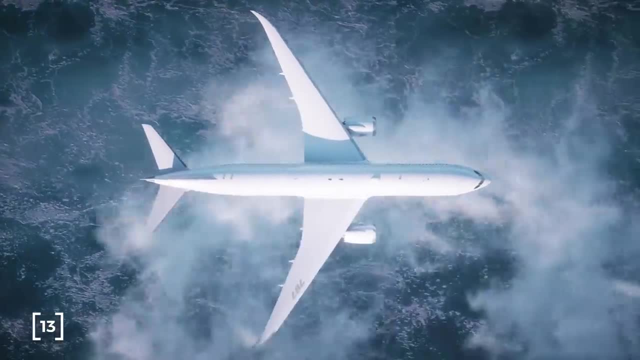 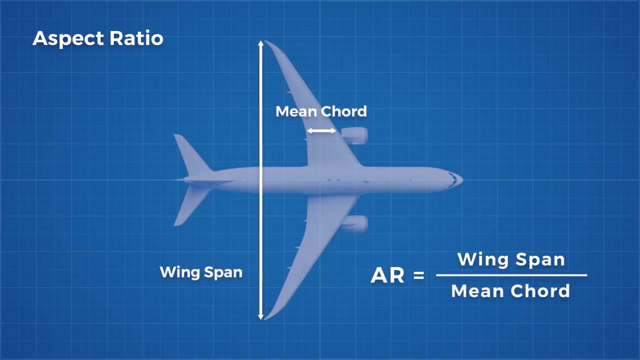 it takes more force to deform the same volume of material But, critically, 787 wings are not the same shape as their aluminium counterparts. This ability to withstand greater bending allowed engineers to make the 787's wings with a much higher aspect ratio. Aspect ratio is the ratio between the wingspan and the mean chord or wing width. A high 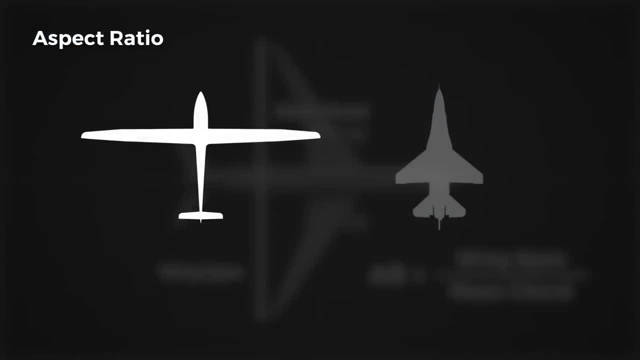 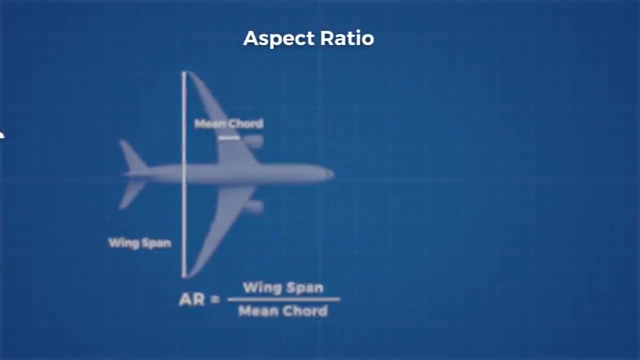 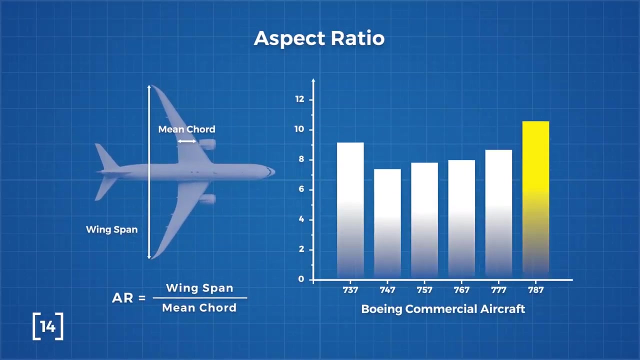 aspect ratio would be a long skinny wing like a glider, while a low aspect ratio would be a delta wing of a fighter jet. A traditional airliner has an aspect ratio of about 9,, like the 787's predecessor, the 777, but the 787 has a massive aspect ratio at 11.. This 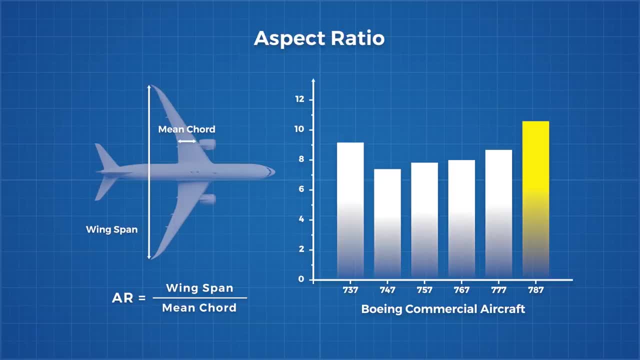 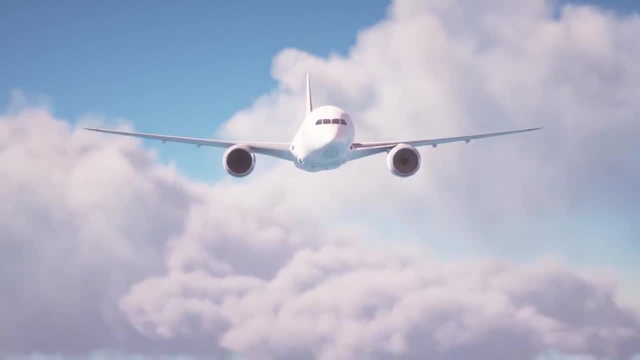 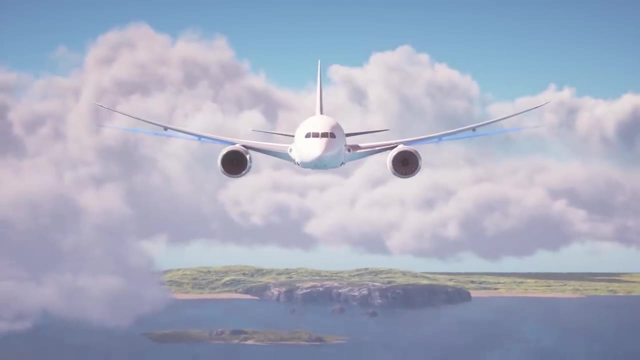 is what causes the 787's wings to flex so much during flight. Composites are actually stiffer than aluminium, but their ability to withstand high deformation allowed the engineers at Boeing to create a much higher aspect ratio wing- A longer, narrower wing that would bend more, But this comes with some huge benefits. 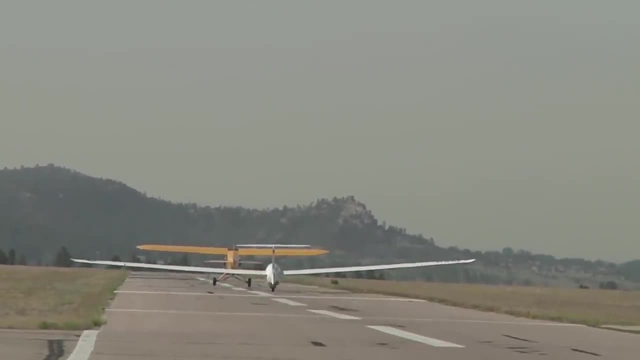 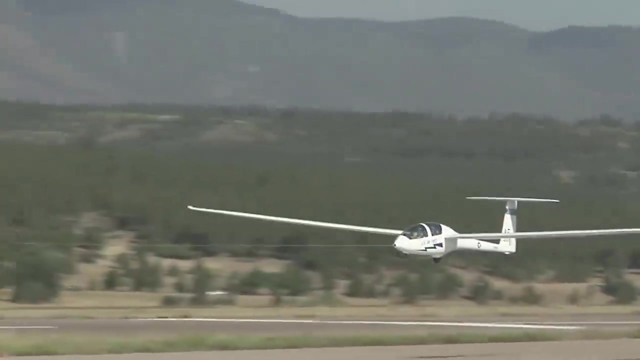 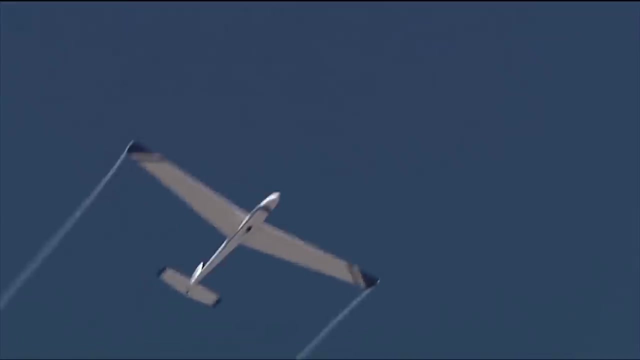 The planes with the highest aspect ratio are gliders. For an unpowered plane, the highest priority is minimising energy lost to drag. This allows the glider to stay in the air for extended periods with no engine. These types of aircraft typically have aspect ratios. 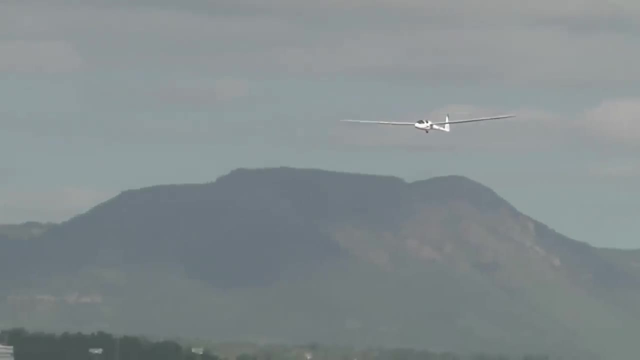 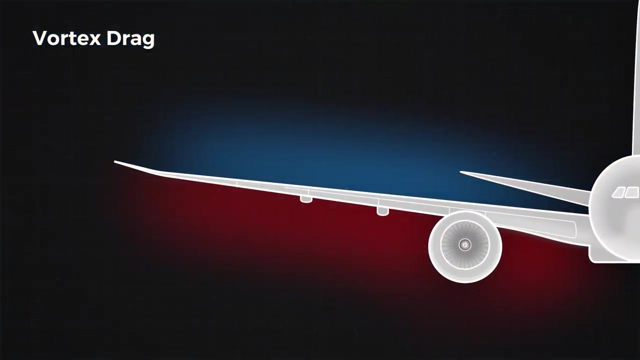 greater than 30, and these aircraft have the lowest drag penalties as a result of vortex drag. This is the drag caused by air mixing from the high pressure zone under the wing with low pressure air above the wing, forming vortices at the wing tip By spreading the 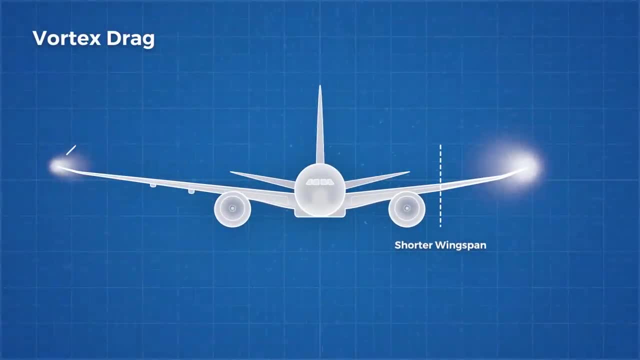 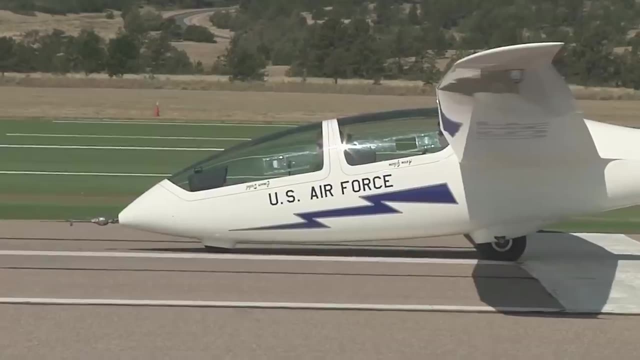 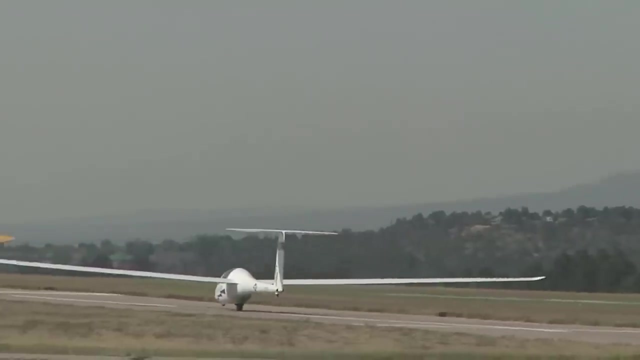 area of the wing over a longer span, we minimise the pressure that drives this mixing at the wing tip and thus minimise the energy lost to the vortices. Normally, higher aspect ratio wings have lower internal volumes. For an unpowered glider, this isn't an issue. But 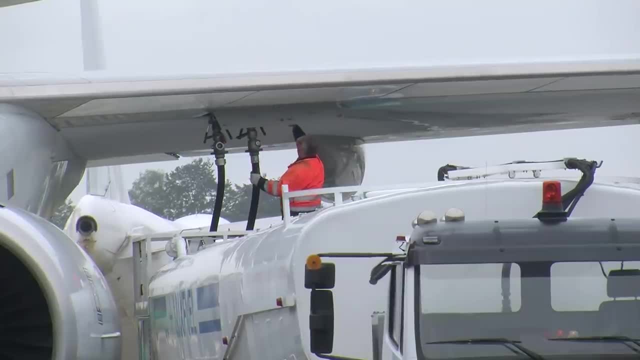 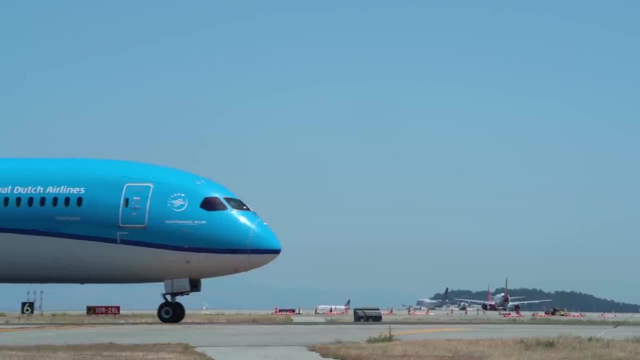 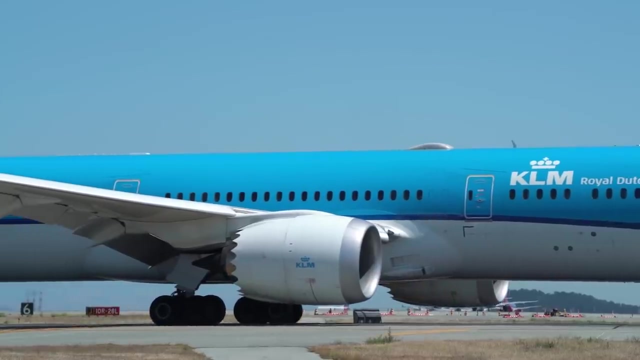 for a plane that needs that storage space for fuel, it is Less. storage volume for fuel means lower range, and one of the primary goals of the 787 is to be an efficient, long range aircraft capable of allowing airliners to open new routes that were once deemed impossible. 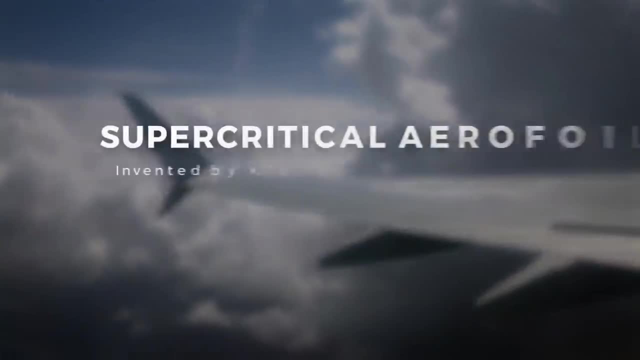 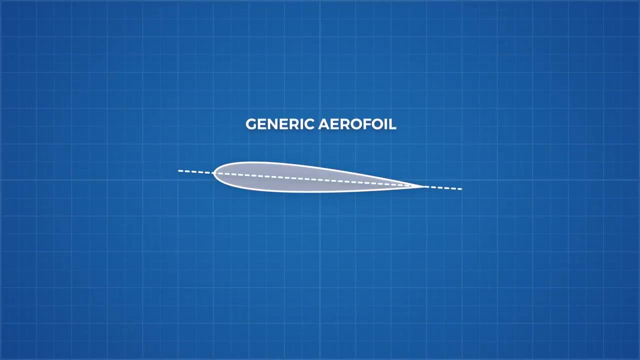 Thankfully, modern planes like the 787 use a new kind of aerofoil, The supercritical aerofoil. Older aerofoils look something like this: A reasonably symmetric design with a sharp nose and gentle curves on the upper and lower surface. And this is a supercritical. 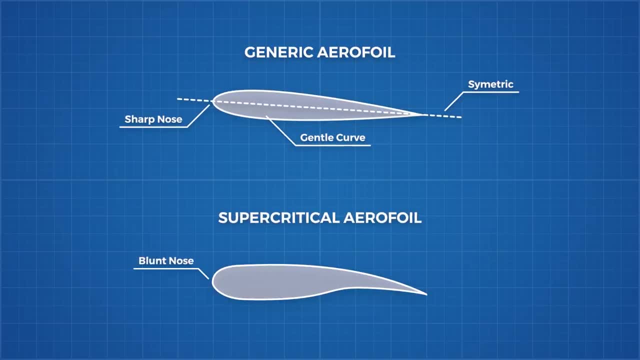 wing. The leading edge is blunter, with a larger radius, the top is relatively flat and the lower portion has this strange cusp at the back. This aerofoil has much more useful internal volume thanks to its blunt leading edge and larger thickness to chord ratio. 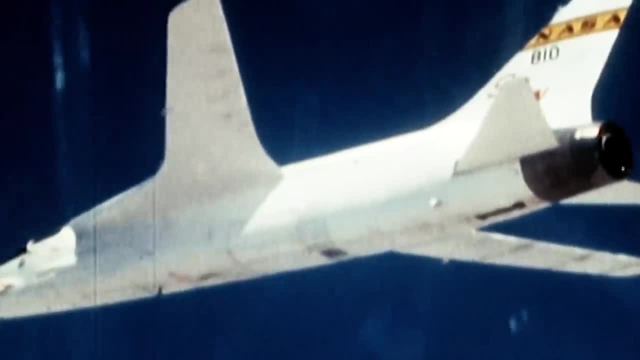 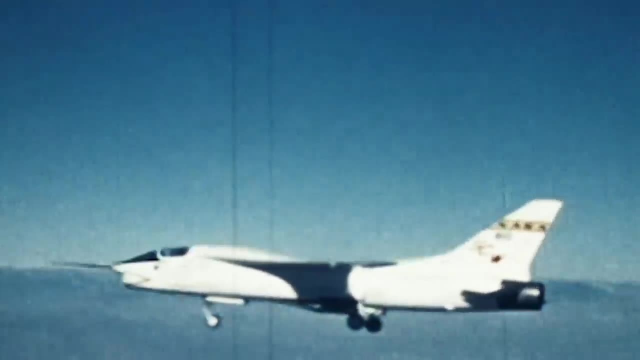 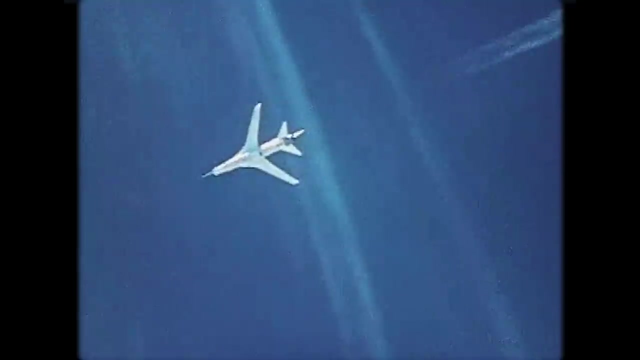 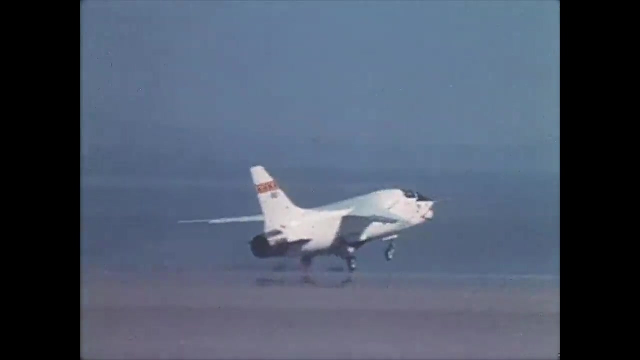 Helping solve our low internal volume problem associated with high aspect ratio wings. the supercritical wing was first tested by NASA on a modified TF-8A Crusader And you can really see the similarities in design ethos between the experimental planes sleek wings with the 787.. But increased internal volume is not why NASA developed the supercritical. 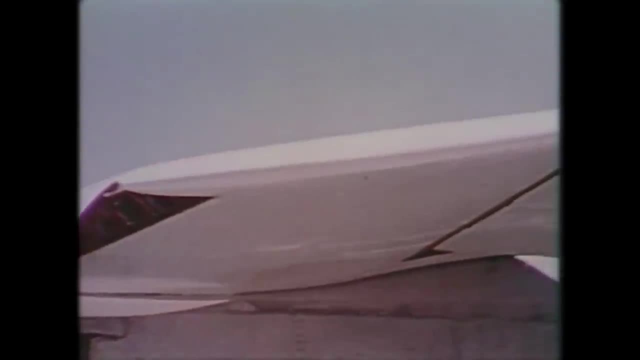 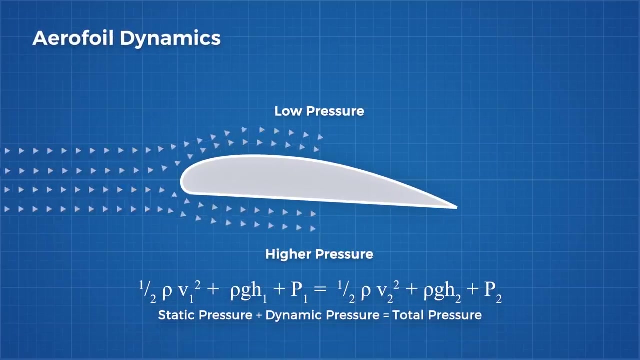 wing. NASA developed it to delay the onset of shockwave formation over the wings. When air travels over a wing, the air on top accelerates. This means that even though the plane itself might be travelling below the speed of sound, The air over the wing may break it and create a shockwave. This shockwave decreases lift. 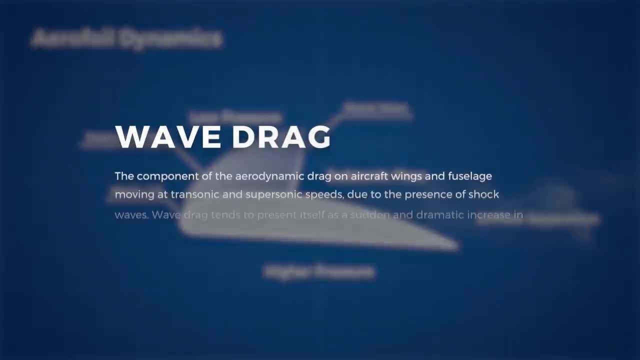 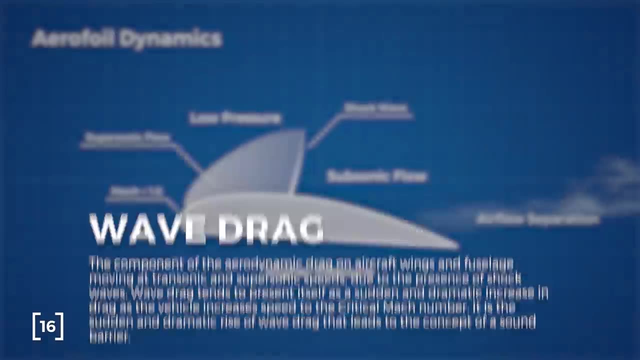 and causes an increase in drag. This kind of drag is called wavedrag and planes need to fly below the speed this occurs at. The speed is called the critical Mach number. The supercritical wing was designed to increase the critical Mach number. The flat top of 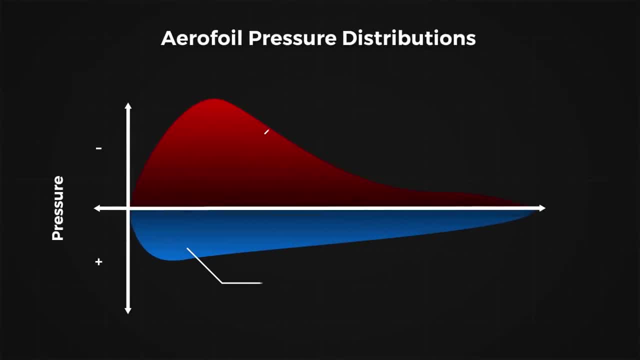 the supercritical wing means the air does not accelerate as much as it would over a classic aerofoil. Of course this causes a loss in lift because that fast moving air is causing a drop in pressure on top of the wing. To compensate, supercritical aerofoils have this concave. 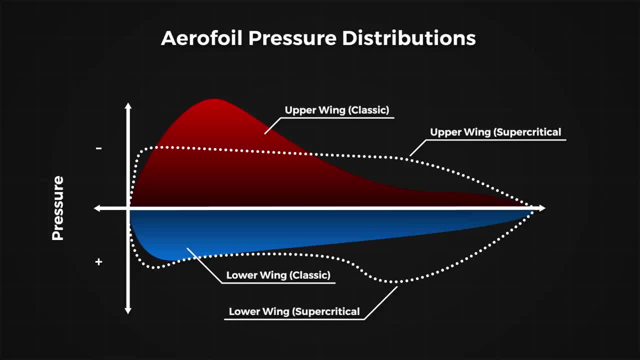 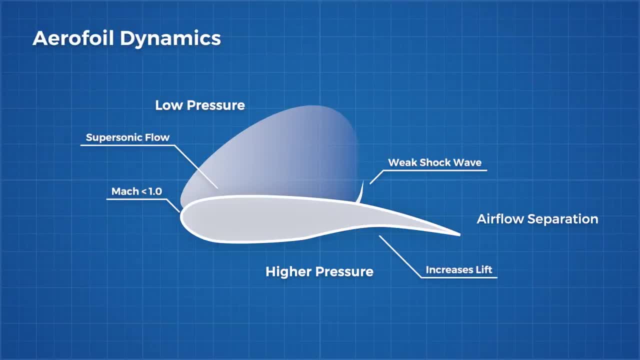 curvature underneath the wing, which causes an increase of pressure there to compensate This increase in pressure does not affect the critical Mach number, While the larger radius of the leading edge increases the lift generated at higher angles of attack. This is because air struggles to follow the tighter turns. 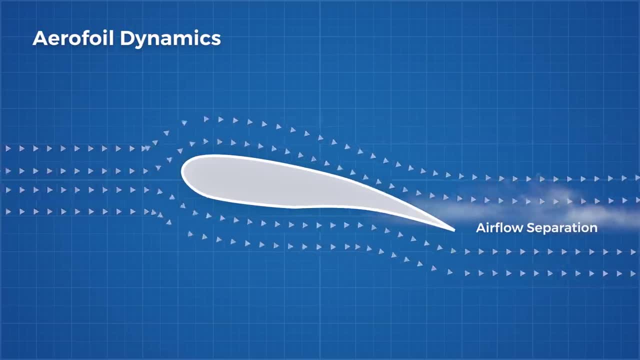 Air also plays a major role in putting pressure into the wing, and this is why the wing is not simply a drop in pressure, but an increase in air pressure. This is why the wing is made turns of a smaller radius leading edge, which causes earlier flow detachment and stall. 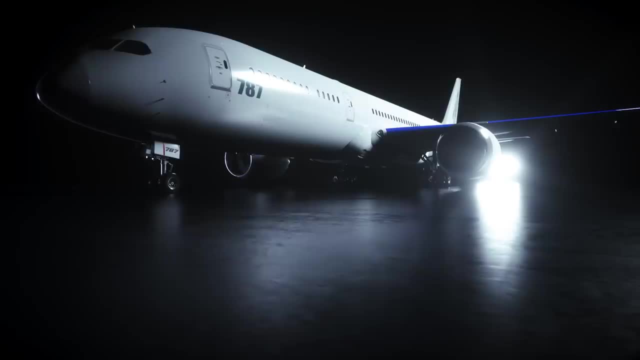 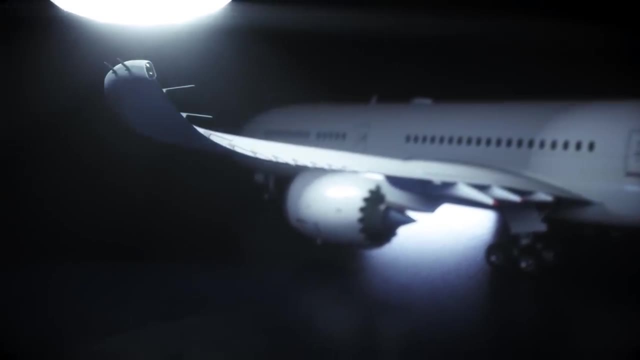 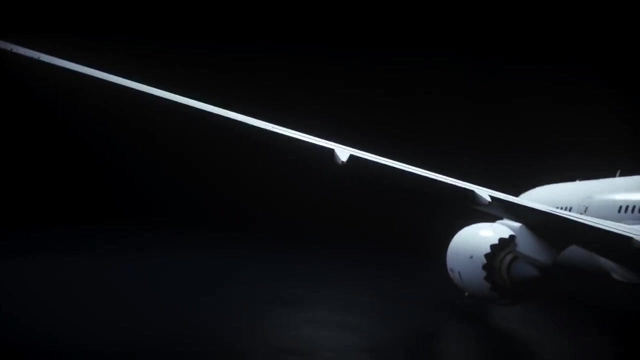 The larger radius delays this flow separation. This aerofoil shape changes continually as you travel: the length of the wing twisting and curving in computer calculated precision, optimising the wings shape to be as efficient as possible and composites, provided the engineers with the confidence that these shapes could. 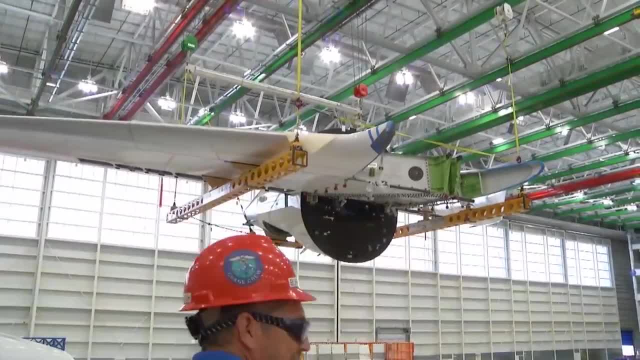 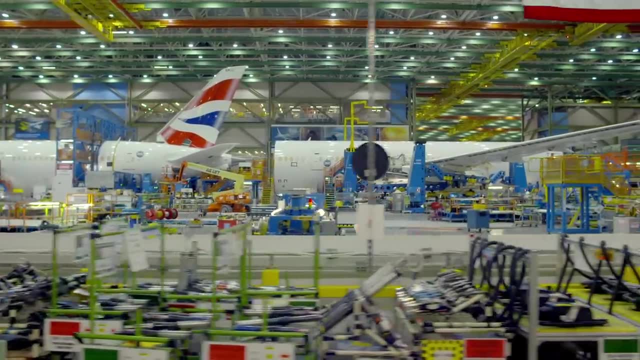 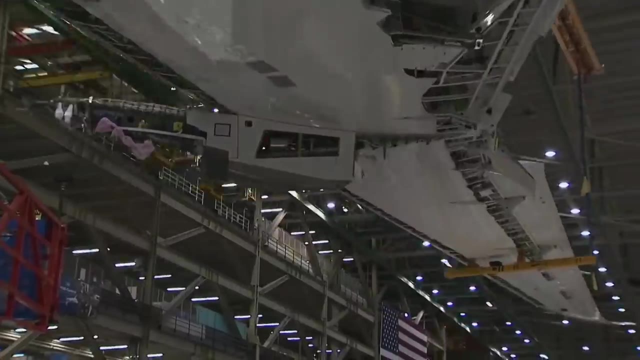 be manufactured. The skin is simply laid down on a mould with automated tape laying. once again, We don't have to beat metal into shape each and every time we want to recreate these delicate curves. The fibres of the wing have even been laid in specific patterns to tailor the stiffness. 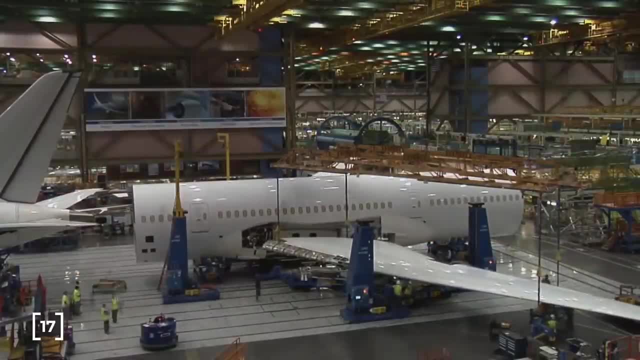 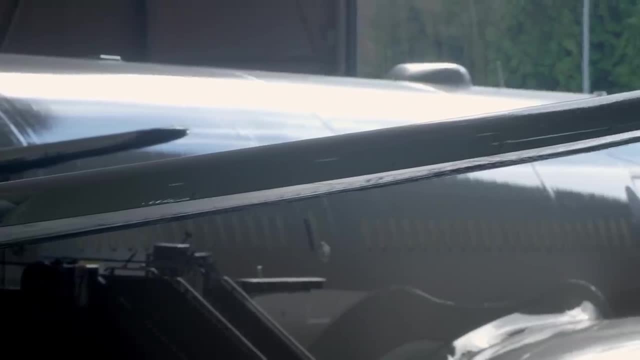 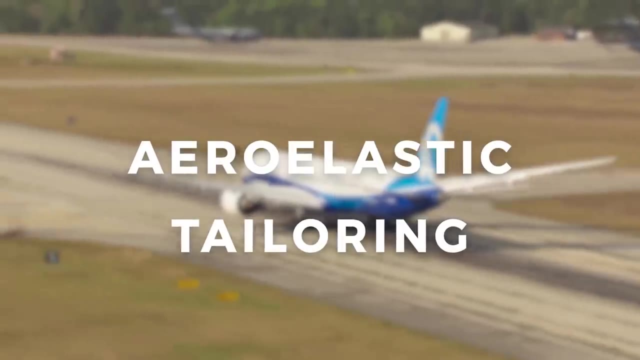 of the wing in different areas. This means the wing deforms exactly as the 787's engineers wanted to as it gains speed. So the wing shape actually changes during flight To better suit the needs at different speeds. This is called aeroelastic tailoring and is the forefront of state of the art aeronautical. 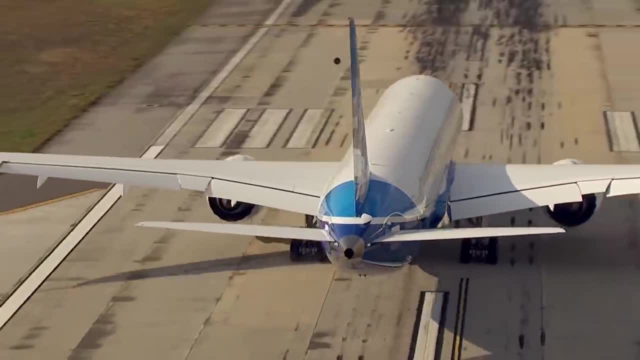 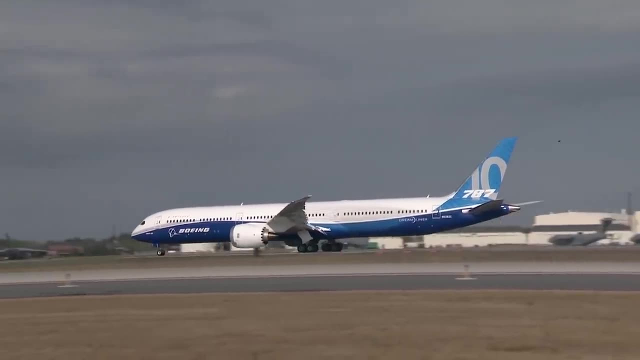 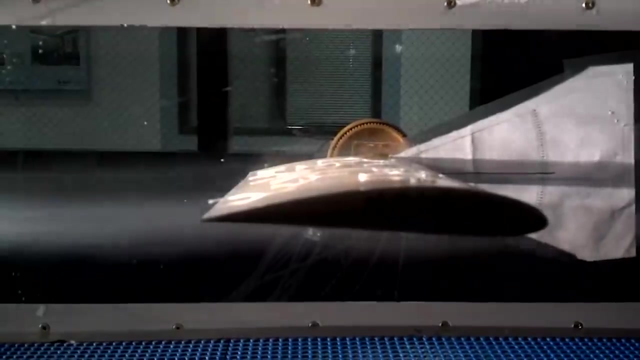 engineering. today, The 787 also features a novel device designed to reduce turbulent flow over the tail of the aircraft. Two types of flow states exist in aerodynamics. Laminar flow occurs at low velocities and is characterised by fluid layers flowing smoothly over each other in neat, orderly layers. 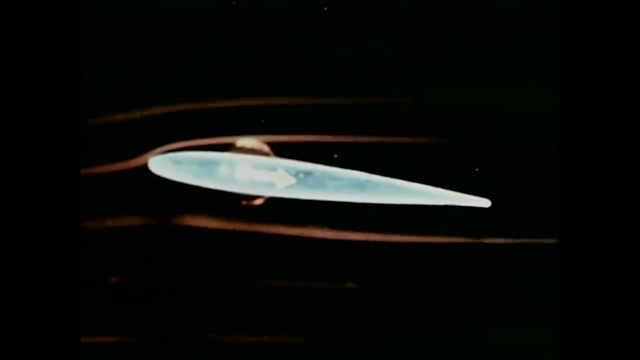 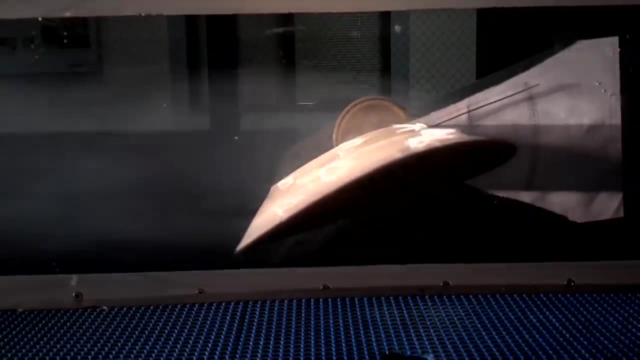 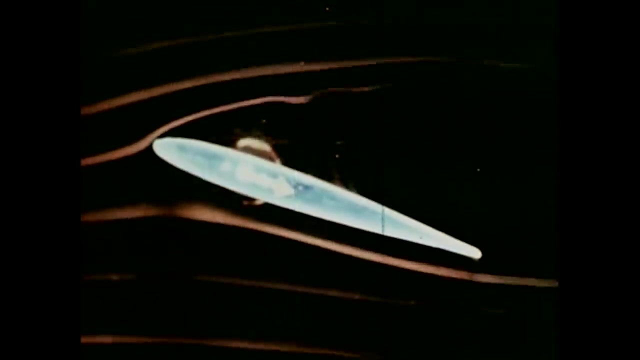 Laminar flow is predictable and non-erratic and does not create significant drag. Turbulent flow is far more common, but still very little is known about how to predict its behaviour. It is very difficult to control because of the formation of small vortices called eddies. 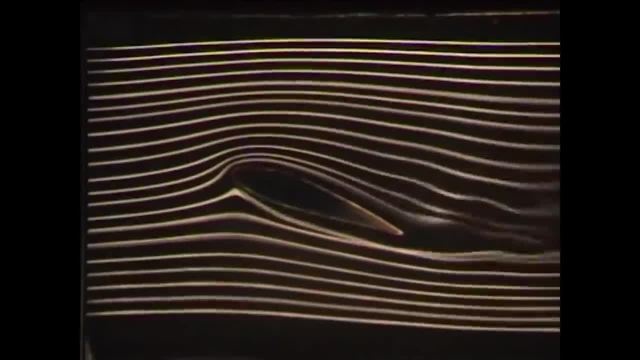 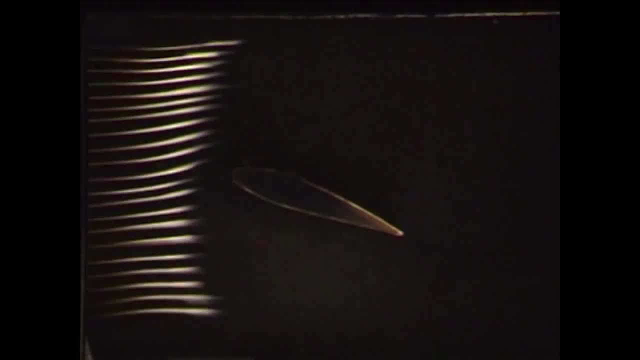 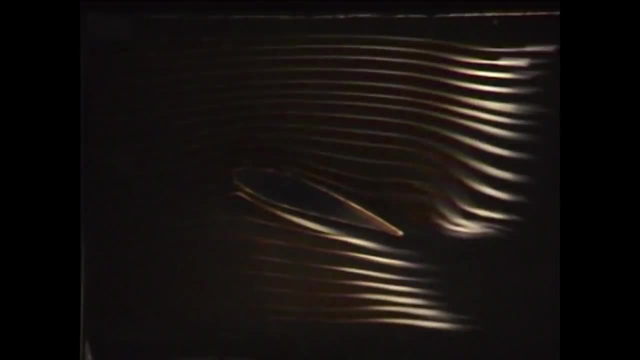 in the flow, making the flow highly erratic. Turbulent flow occurs at higher flow velocities and causes a significant increase in drag At cruising speeds of 80-85% of the time This is a very common phenomenon At speeds of 100% of the speed of sound. turbulent flow is ultimately unavoidable, but we can. 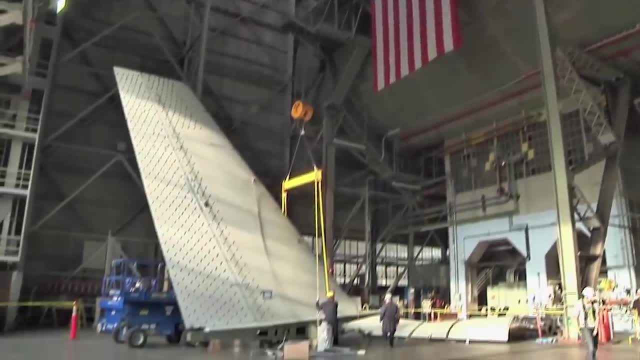 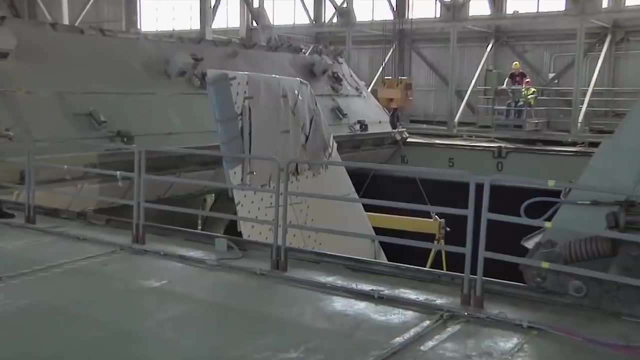 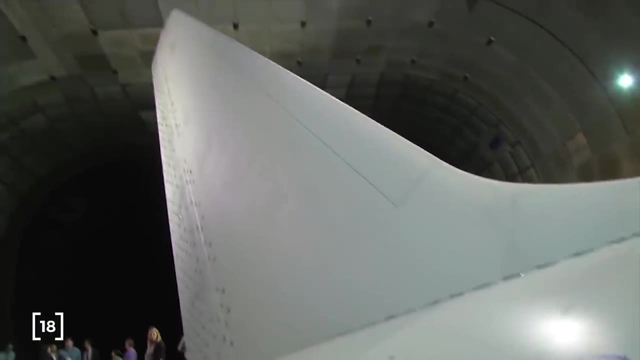 work to minimise it. Boeing has developed a technology that helps them delay and control the formation of turbulent flow, called hybrid laminar flow control. Details on their implementation of the technology are sparse. This technology is capable of reducing fuel burn by as much as 30%, and so companies are. 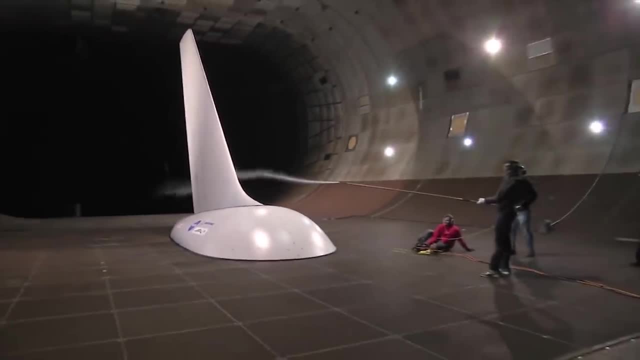 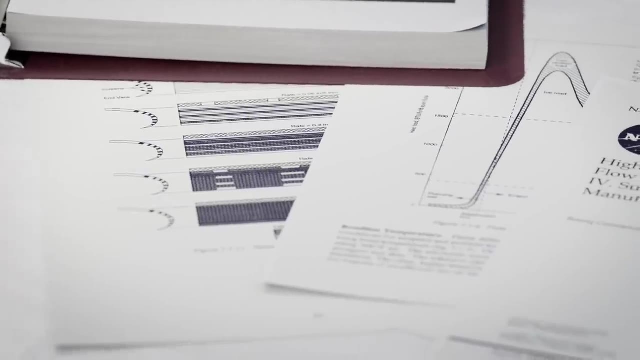 keeping their research extremely secretive to keep their competitive advantage. This technology is capable of reducing fuel burn by as much as 30%, and so companies are keeping their research extremely secretive to keep their competitive advantage. Here's what we know. In the late 80's and early 90's, NASA and Boeing began investigating a suction system. 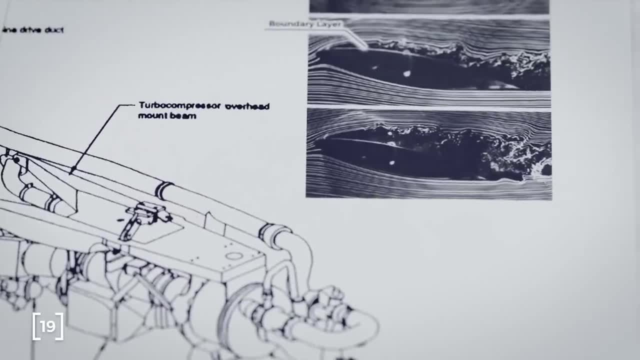 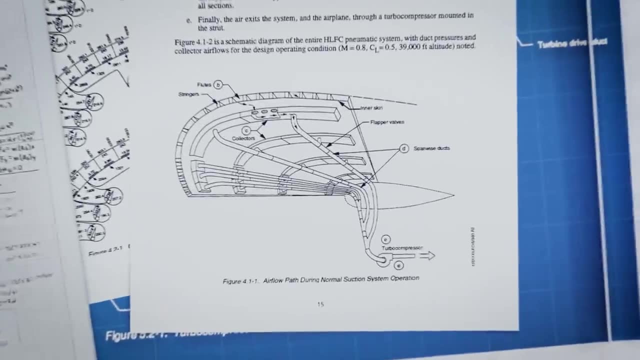 on the 757 that would draw in boundary layer air, That is, the layer of very slow moving air that clings to the surface of moving objects. The outside skin was permeable to air through tiny perforations too small for the naked eye to see. 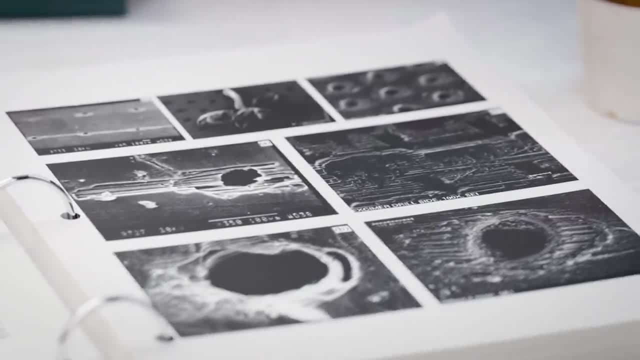 Manufacturing the permeable surface while also keeping the tiny holes clear of debris is one of the most important things to keep the surface clean. The surface is made up of a layer of air that is permeable to air through tiny perforations too small for the naked eye to see. Manufacturing the permeable surface while also keeping the tiny holes clear of debris is one of the most important things to keep the surface clean. The surface is made up of a layer of air that is permeable to air through tiny perforations too small for the naked eye to see. 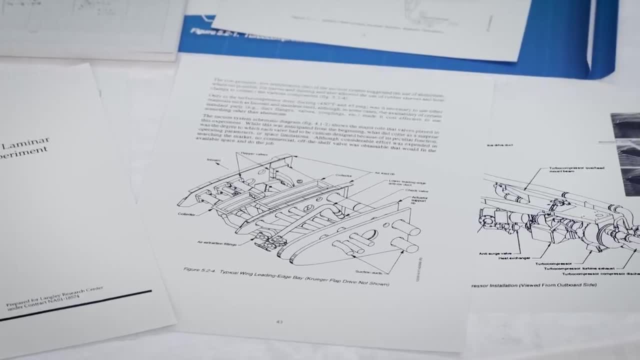 The surface is made up of a layer of air that is permeable to air through tiny perforations too small for the naked eye to see. Manufacturing the permeable surface while also keeping the tiny holes clear of debris is one of the most important things to keep the surface clean. 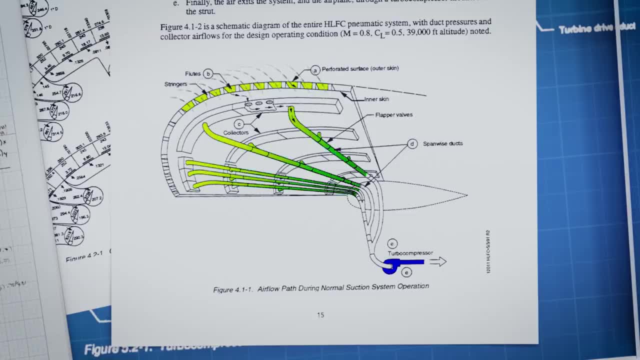 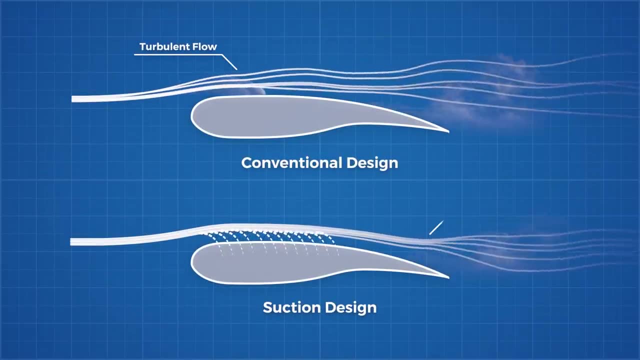 The outer and inner skin were then attached to an elaborate plumbing system that was connected to a turbopump, which sucked air from the boundary layer of air that would form along the plane's surface. By doing this, they could drastically delay and reduce the size of the turbulent flow. 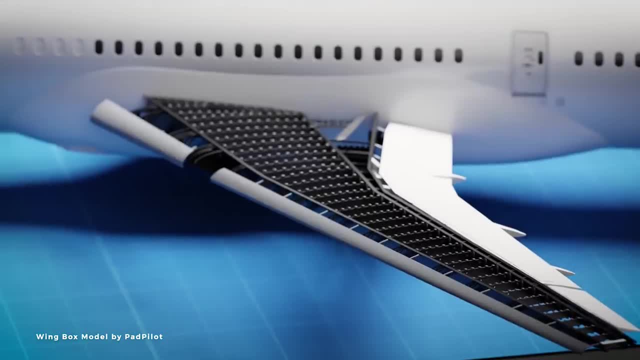 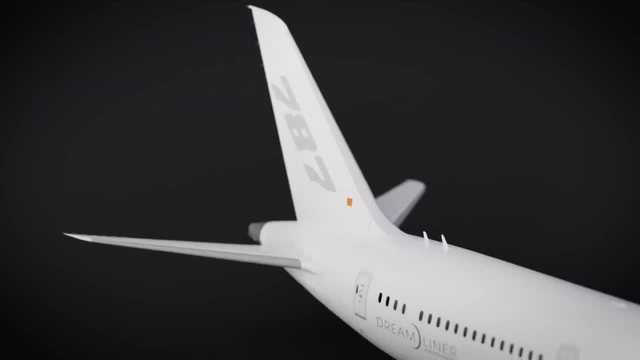 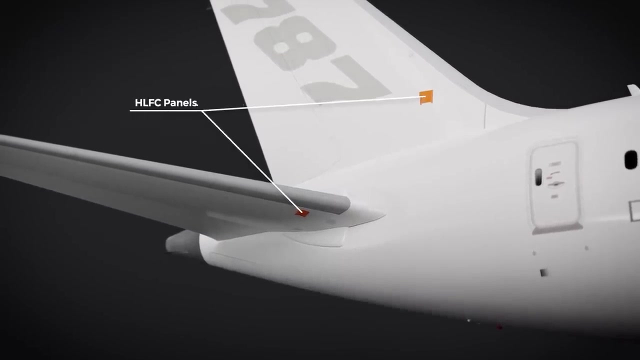 and in turn, reduce the drag on the plane. There is no space for this ducting system inside the wings of the 787, but from what we do know, it is inside both the horizontal and vertical tails. However, the only clue of their presence are these tiny doors whose purpose are a mystery. 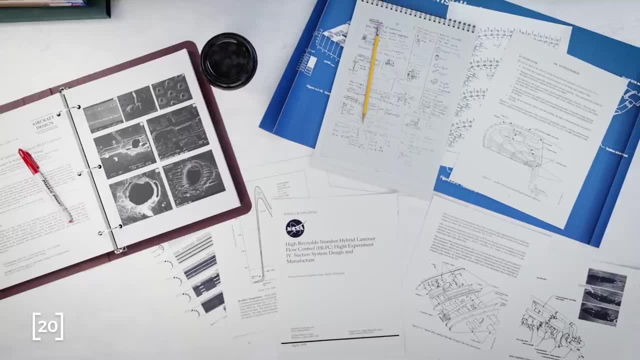 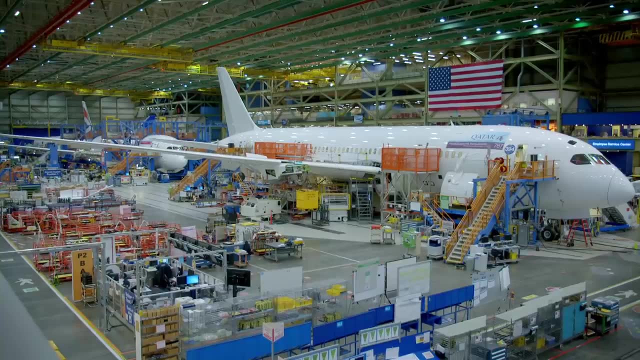 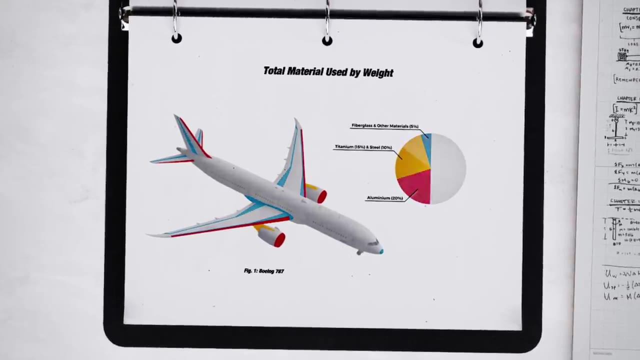 to me, with little to no information available online, a testament of how advanced this plane is. Composites give plenty of advantages, but it does come with some disadvantages. When we examine the plane's composition, one material jumps out at me: 15% of this plane is titanium. 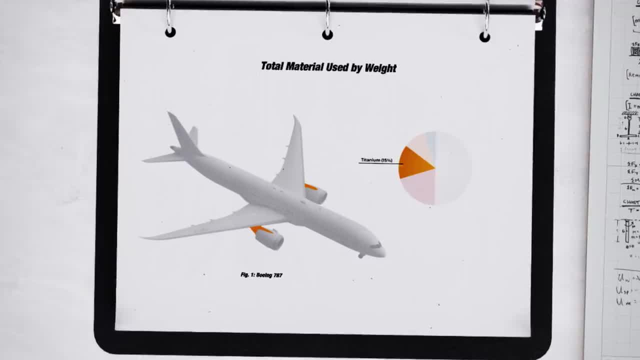 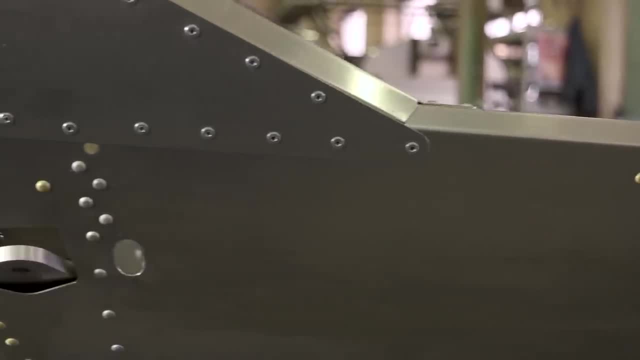 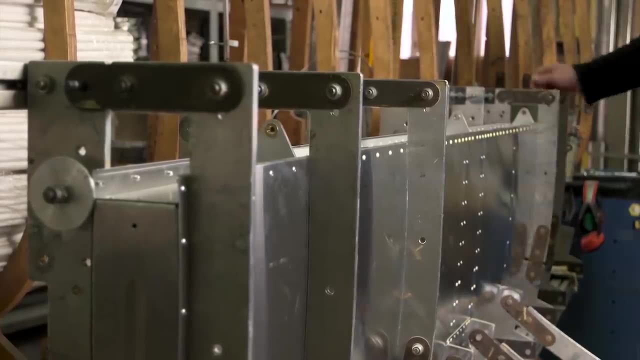 That's much higher than normal. Titanium is an expensive material, so they must have had a good reason to use it over aluminium. Aluminium is typically corrosion resistant when it's left on its own, but when it is placed in direct contact with carbon fibre composites, something strange happens. 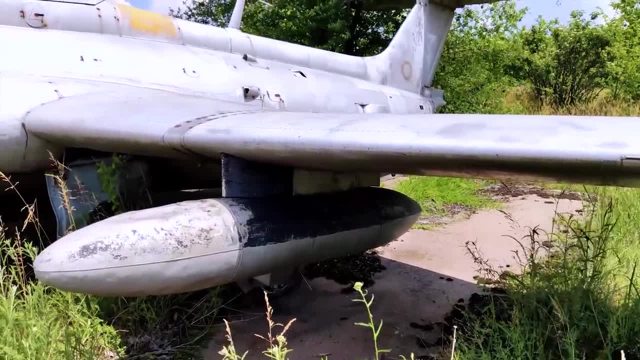 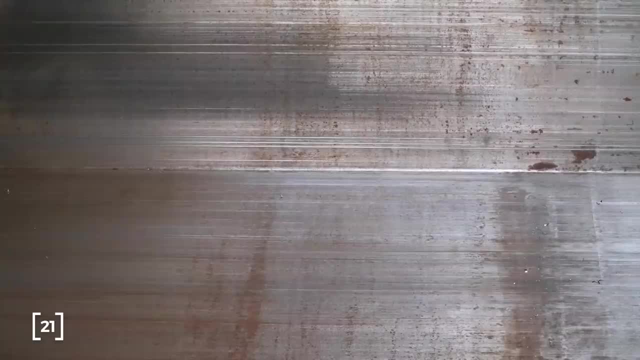 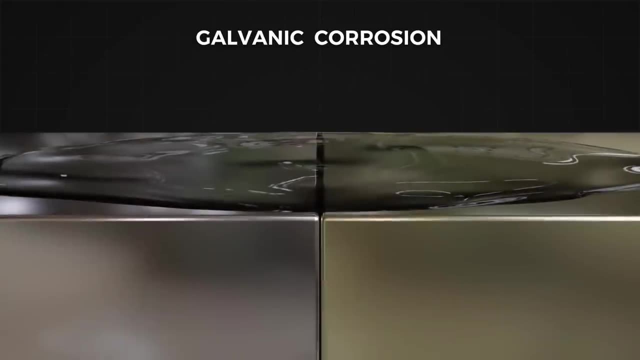 The aluminium begins to corrode incredibly quickly. Something about carbon fibre causes aluminium to oxidise and fall apart. Carbon fibre is, like aluminium, Aluminium's kryptonite. This phenomenon is called galvanic corrosion, and it happens when two materials that have 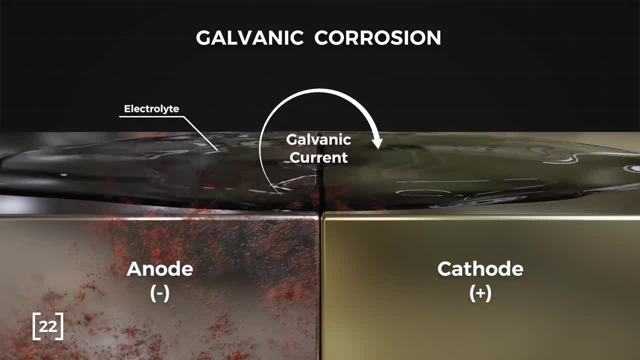 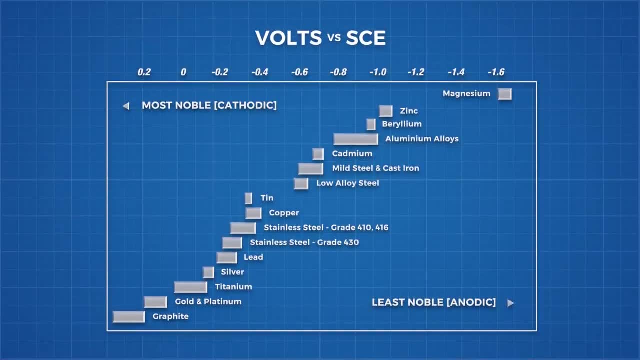 dissimilar electric potentials, or nobilities, are placed in contact with an electrolyte like salt water. If we look at the galvanic series, which quantifies materials nobilities, we can see that graphite is very noble on the far end of the left scale, while aluminium is quite far to the 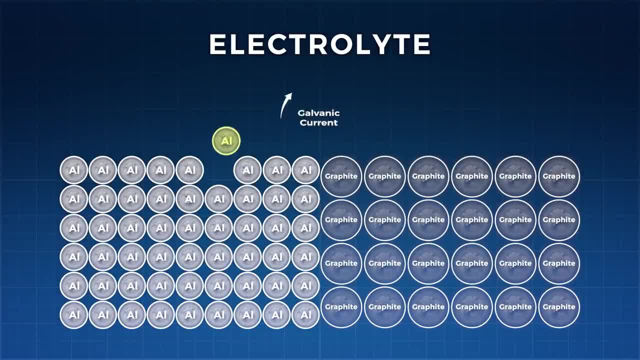 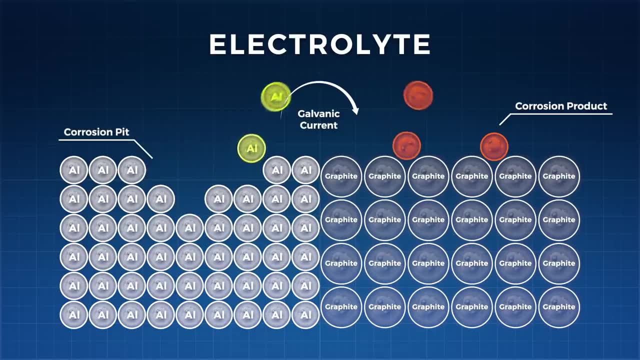 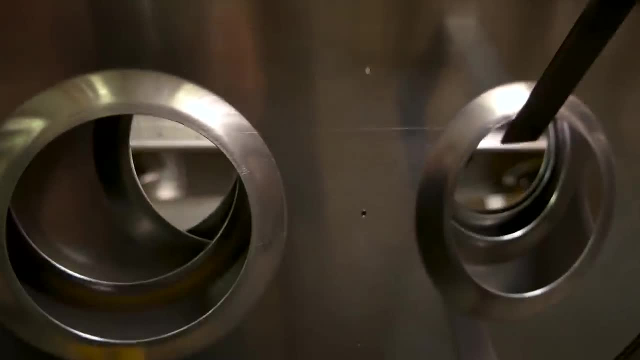 right, Aluminium occurs and electric potential forms between the two materials. that causes the two materials to trade electrons and ions, which results in the anode being eaten away. This effect is made even worse when the surface of the more noble material, the cathode, is. 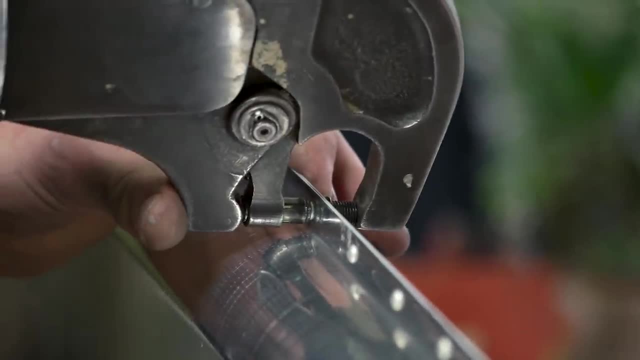 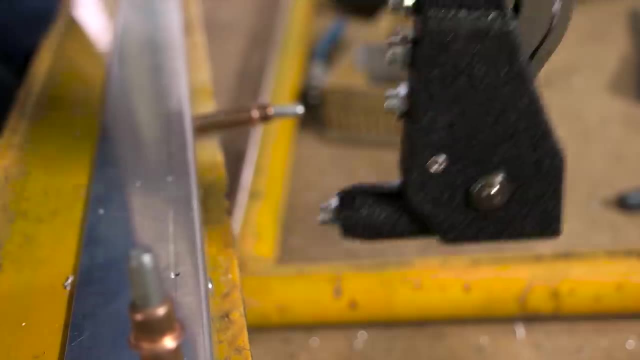 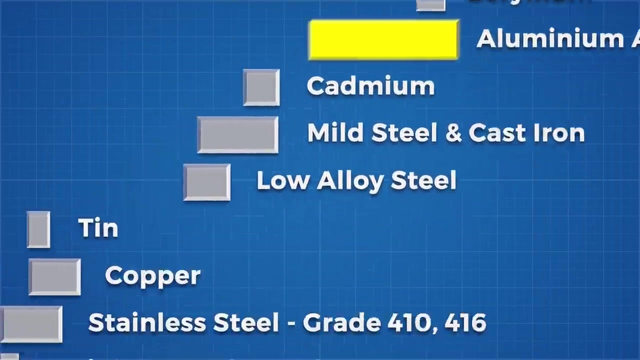 very large in comparison to the less noble material, the anode Say. for example, when carbon fibre composites are fastened together using aluminium fasteners. To avoid this corrosion, the engineers needed to pick a material closer to carbon in the galvanic series, and the closest suitable metal was titanium. 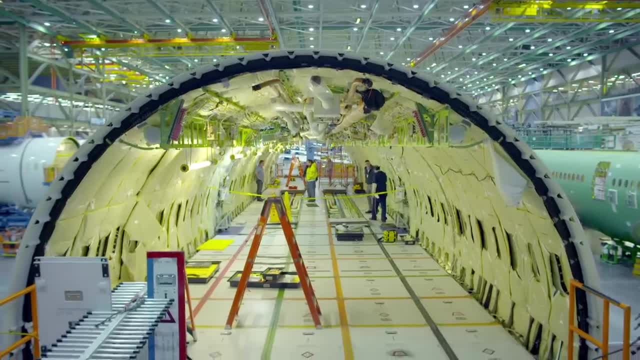 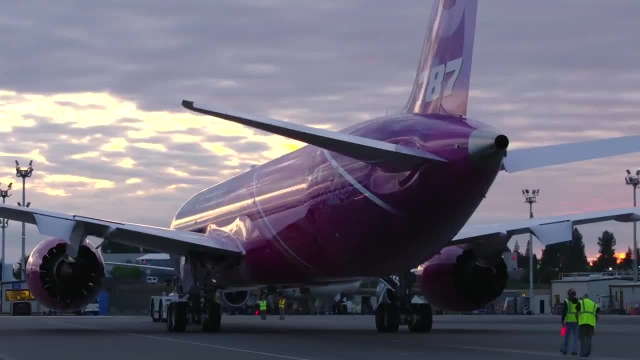 This has been a huge source of cost in manufacturing. Boeing's production cost was higher than its sales price for quite some time, Meaning they were making a loss on each aircraft sold. This is fairly typical for new airliners, as R&D and manufacturing tooling costs take. 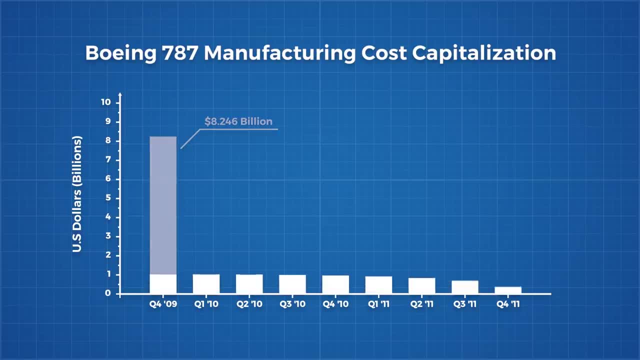 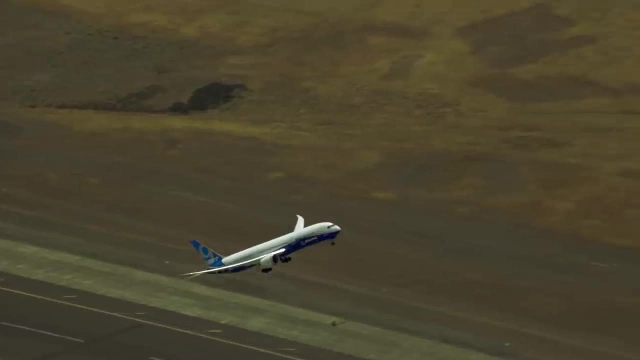 time to recoup And companies like Boeing and Boeing Typically spread these costs over a period of time on each plane instead of just having a massive negative balance sheet in one year. But because the 787 was so radically new, these sunk development costs called deferred. 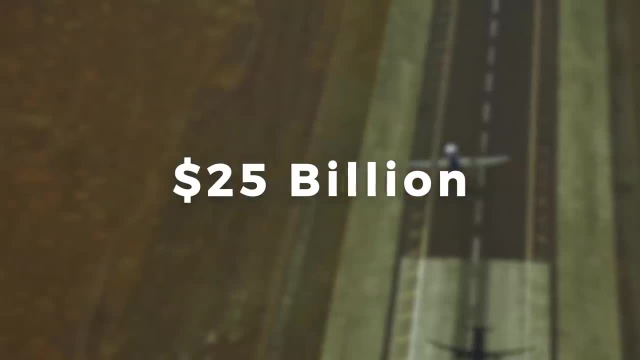 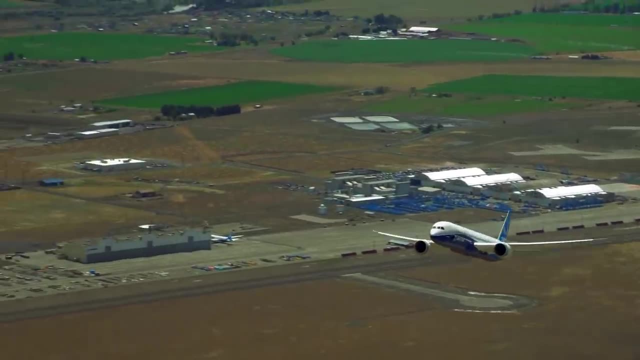 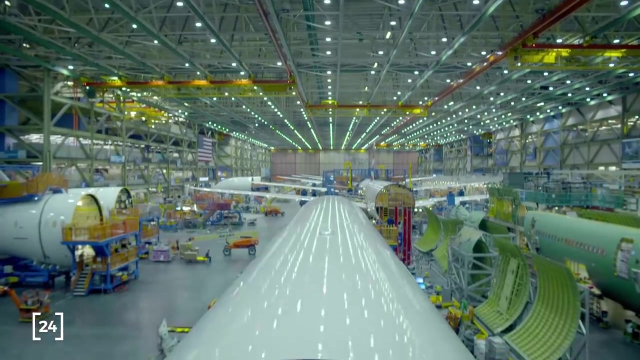 costs were expected to reach 25 billion before Boeing even reached a break even point on each plane sold Where the cost of manufacturing equaled the sales price. In comparison, The Boeing 777 reached 3.7 billion. To recoup costs as fast as possible, it was essential that Boeing reduce the cost of production. 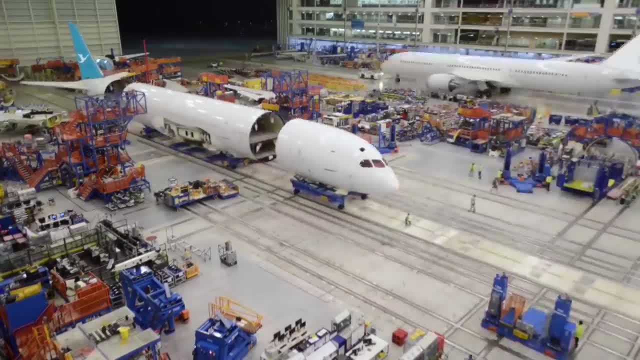 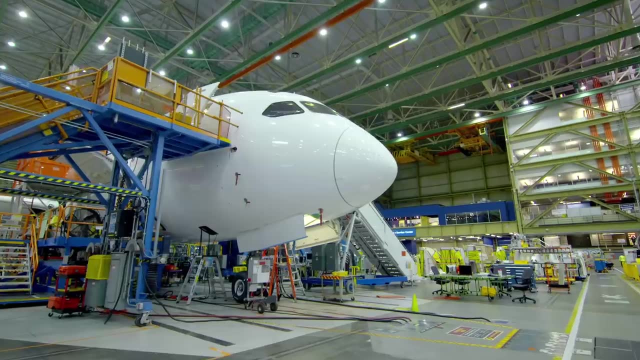 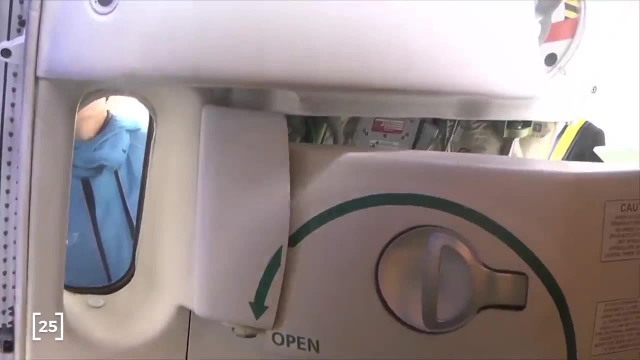 And high on their list was the elimination of titanium parts where possible. The frame around the cockpit windows, for example, were initially made out of titanium but were changed to aluminium with a special coating to prevent corrosion, While some parts that were originally titanium were changed to composites, like the door frames. 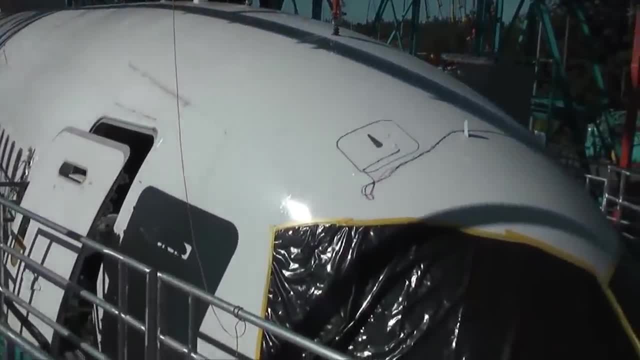 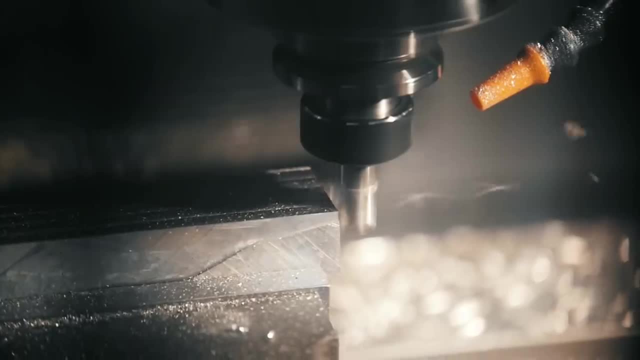 Other parts were changed to aluminium with a special coating to prevent corrosion. While some parts that were originally titanium were changed to composites, like the door frames, Other improvements were sought to make the manufacturing process for titanium less costly. Many metallic parts used on aircraft start off as large blocks of metal that have to 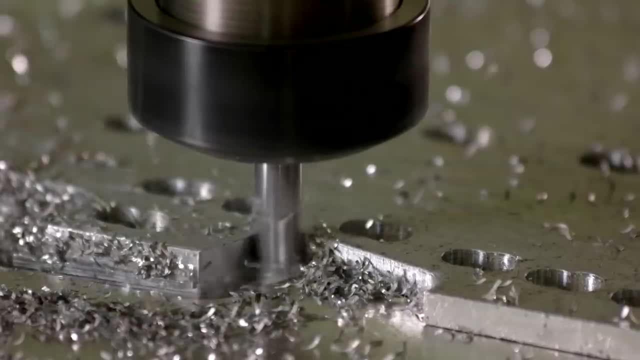 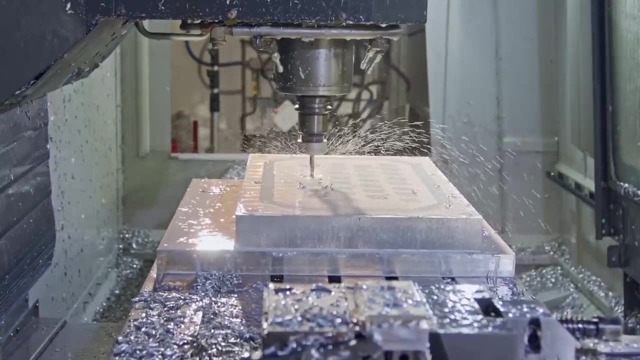 be machined down into their final shape. This results in a tonne of wasted metal, as the metal is gradually shaved away. Aircraft manufacturers quantify this wastage with something called a buy to fly ratio, and it's a huge source of increased manufacturing costs. 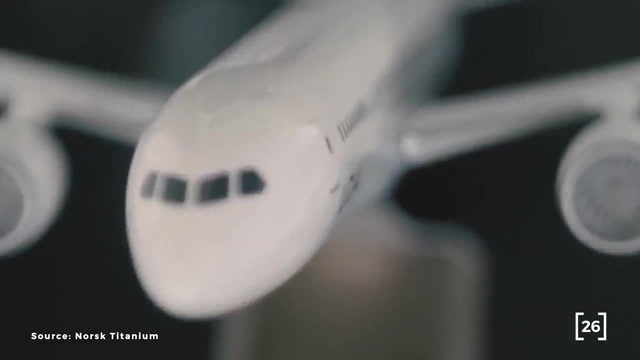 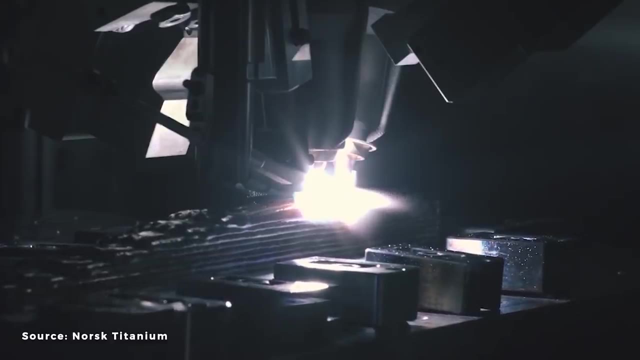 Boeing has tackled the cost of manufacturing of titanium in the past. The cost of manufacturing of titanium in the past has increased But Boeing has tackled by collaborating with Norsk Titanium, a titanium 3D printing company. Now making 3D printed metal parts is not easy. 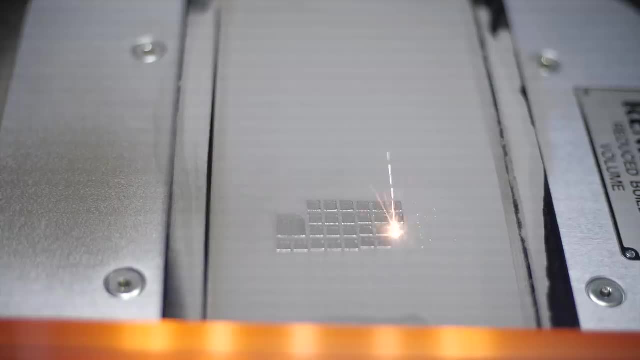 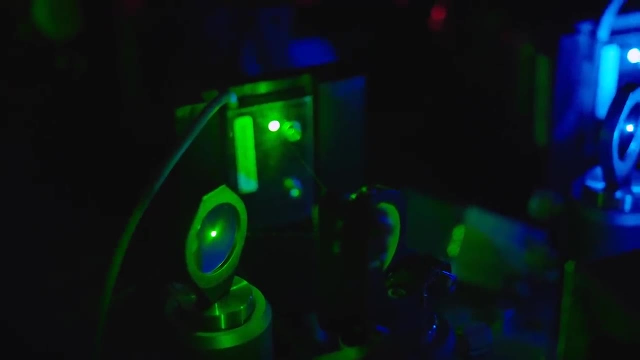 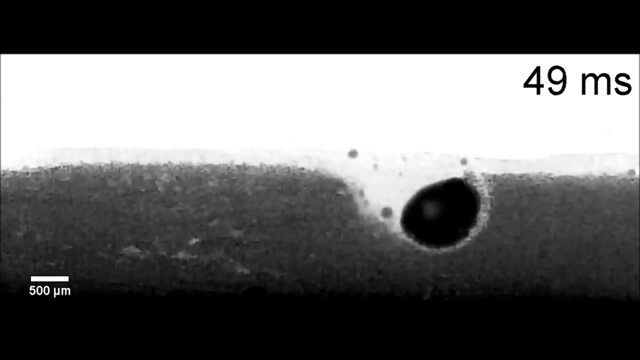 Most titanium 3D printing involves a powdered titanium that is melted together using lasers. Researchers used high speed x-ray imaging to visualise what happens during this process and found a lot of imperfections. The track varies in height. the powder gets blasted away, resulting in varying thickness. 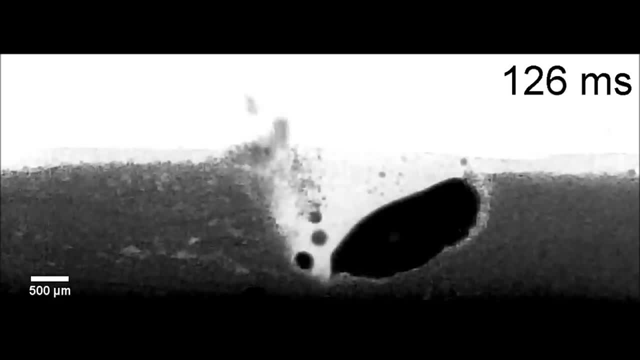 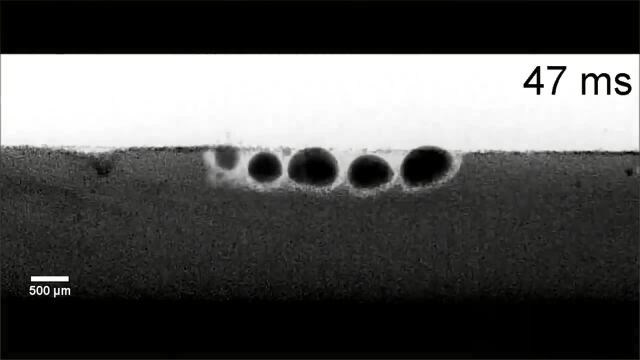 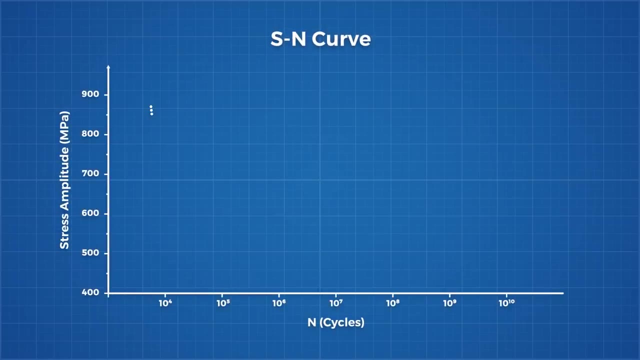 The metal is then separated into separate tracks and even bubbles form, causing pores in the metal. This creates parts with a lot of micro imperfections, and imperfections lead to decreased life as fatigue causes cracks to form. We can visualise a material's fatigue strength by plotting on an SN curve which places the 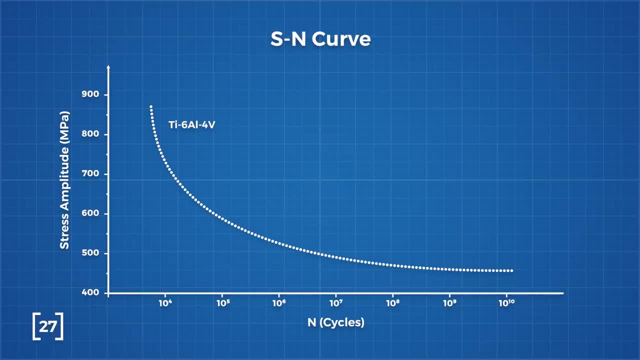 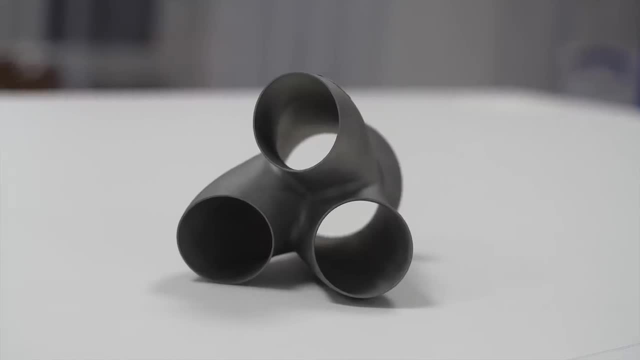 magnitude of the alternating stress on the y-axis and the number of cycles it survived on the x-axis. For example, machined titanium, it looks something like this, whereas for 3D printed parts it looks like this: 3D printed parts simply fail much sooner because of these tiny imperfections. 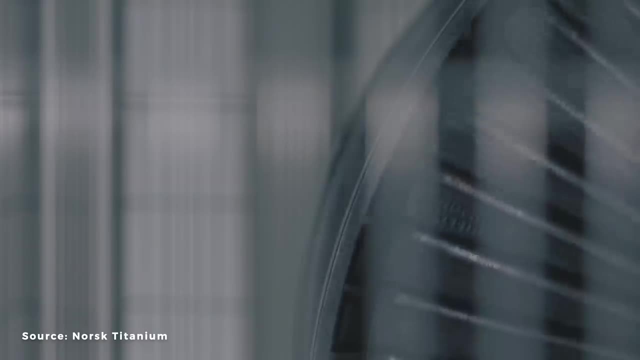 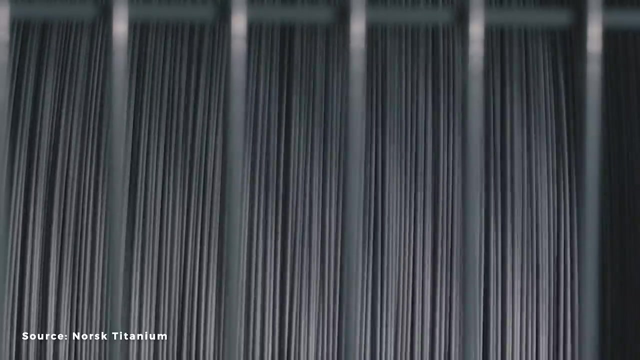 Norsk has worked to improve this. Instead of using laser sintering with powder, Norsk have developed a revolutionising patented wire based metallic 3D printing system for titanium that they monitor with 600 frames per second. cameras for quality control. Norsk has developed a revolutionising patented wire based metallic 3D printing system for titanium that they monitor with 600 frames per second cameras for quality control. Norsk has developed a revolutionising patented wire based metallic 3D printing system for titanium that they monitor with 600 frames per second cameras for quality control. 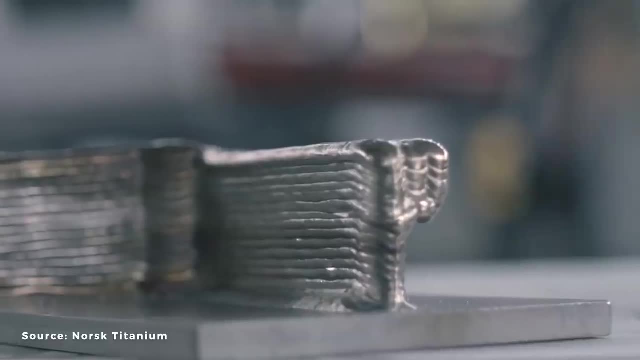 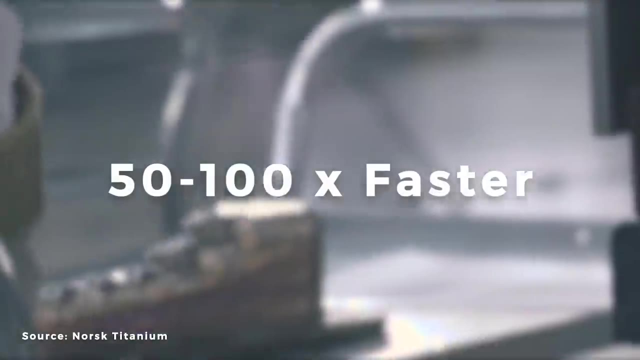 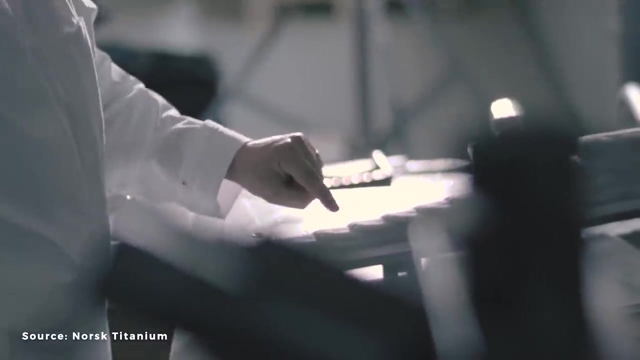 These 3D printed parts are then machined down into their final shape, reducing the total titanium used by 25-50%, and their printing method is 50-100 times faster than the powder printing method. This process resulted in the first ever FAA certified 3D printed structural components. 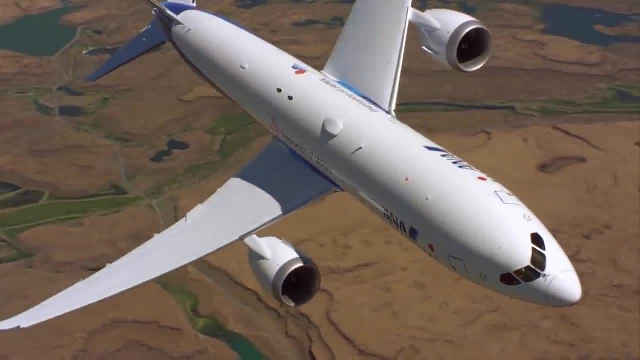 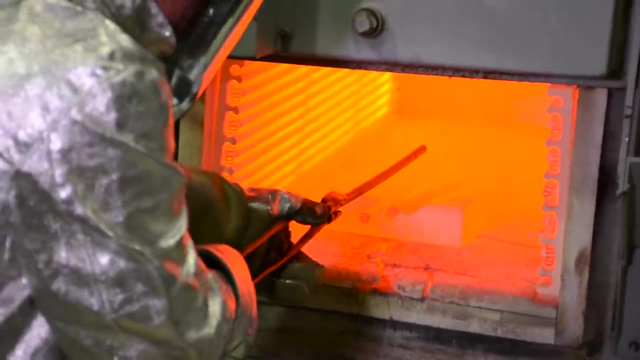 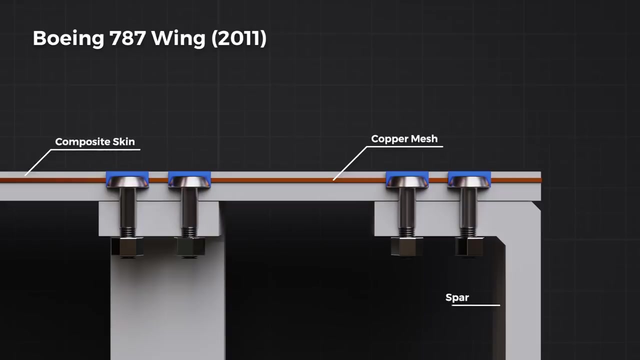 and they first flew in the Boeing 787.. This plane is truly innovative. 3D Printing System for Titanium, Not the only material Boeing worked on removing from the plane's construction to save on cost. Copper once formed an important part of the 787's wing, where it was laid down in thin. 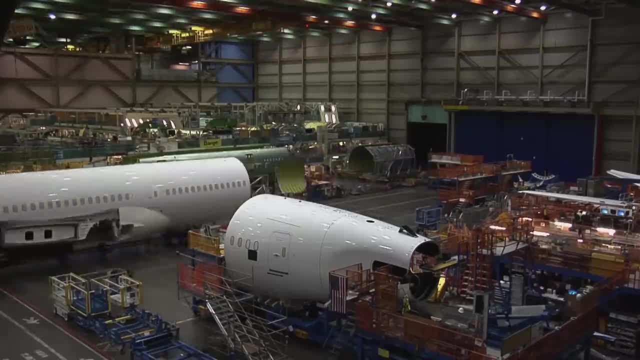 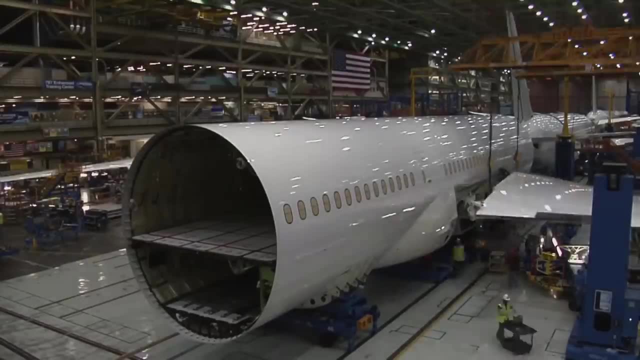 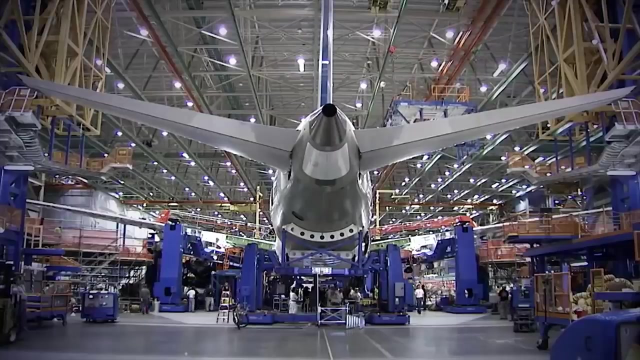 strips on the wing's surface. This is not a typical design choice for aircraft wings and once again it was influenced by the 787's composite construction, because composite materials are not good conductors. Carbon fibres are great conductors, but problems arise. 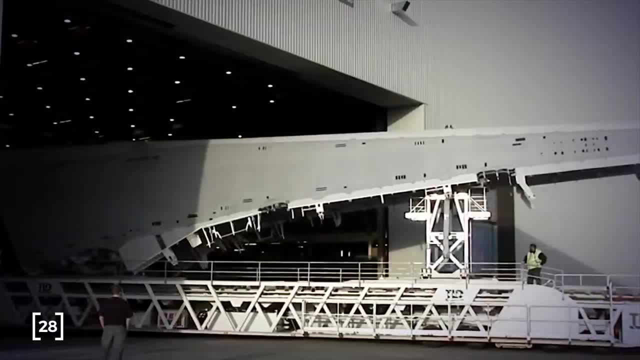 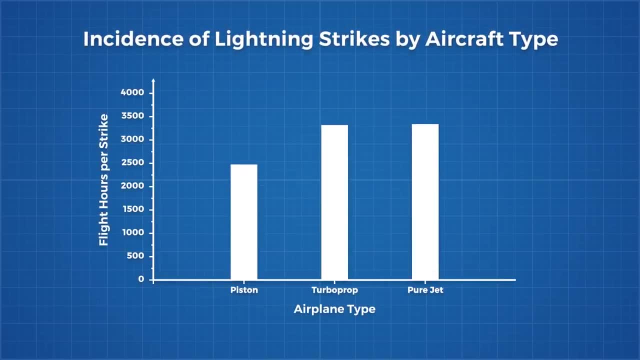 This is because of the plastic resin binding them together, as this resin is an insulating material preventing the passage of electricity, Which is a massive problem for planes, as getting hit by lightning is not a rare occurrence: One study calculated that lightning strikes occurred once every 3,000 hours of flying. 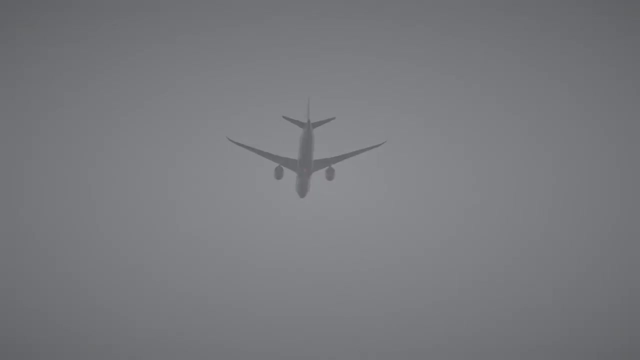 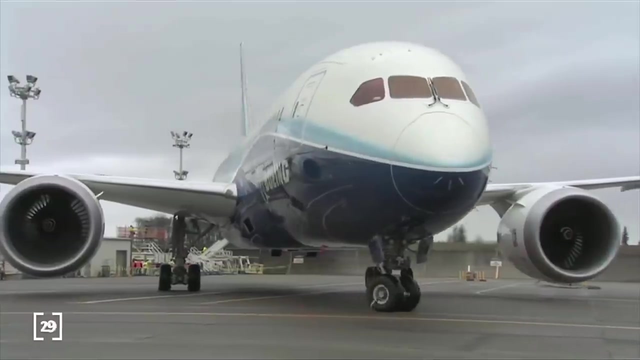 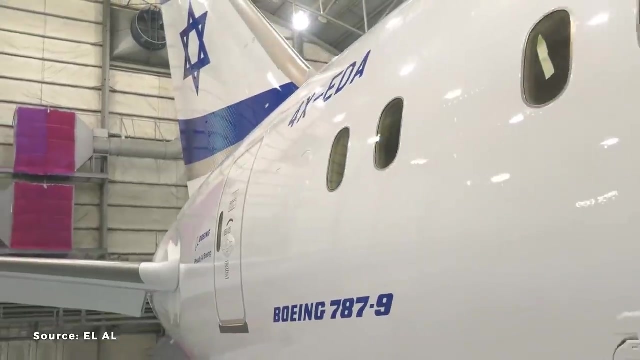 between 1950 and 1975.. A 787 was struck by lightning while taking off from Heathrow. Upon landing in India, 32 to 46 holes were found in the fuselage as a result of resistive heating. The plane survived and was flown back to London for repairs with no passengers aboard. but 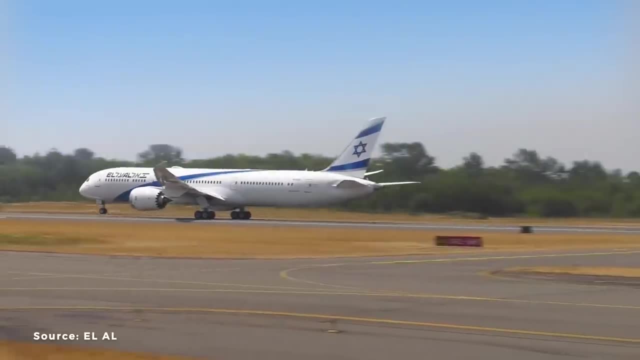 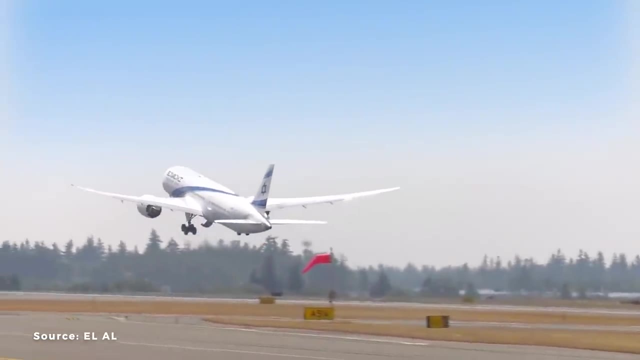 composites, vulnerability to this kind of damage is a drawback, and the repair process is more complicated than with aluminium. However, this strike could have been much worse If the electricity does not run smoothly along the surface of the plane and exit it may. 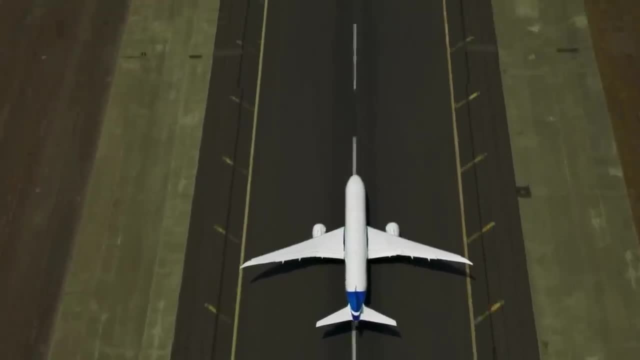 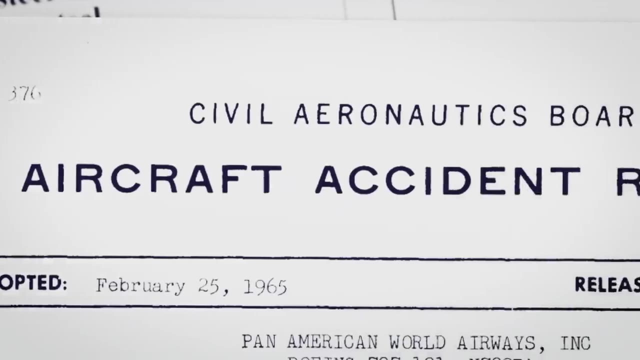 cause a spark in the fuel tanks. This could have been the cause of the fire. This kind of accident was not uncommon in the early days of the airline industry. Pan Am flight 214 was struck by lightning while it flew in a holding pattern waiting. 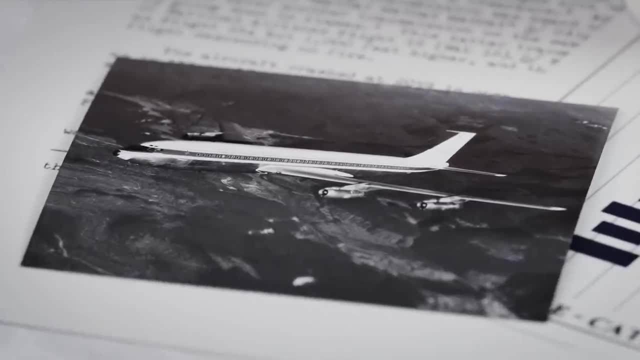 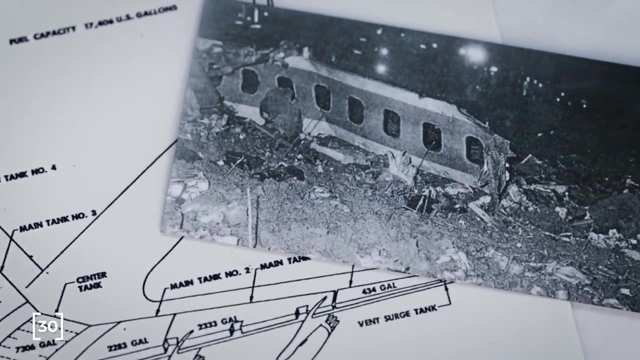 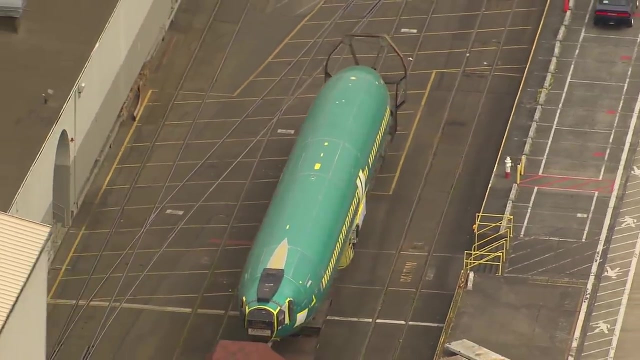 for a lightning storm to pass at Philadelphia International Airport in 1967. It's left wing fuel tank exploded, causing the plane to barrel out of control to the ground in flames. Since then, the aviation sector has implemented rigorous safety measures and lightning protection. 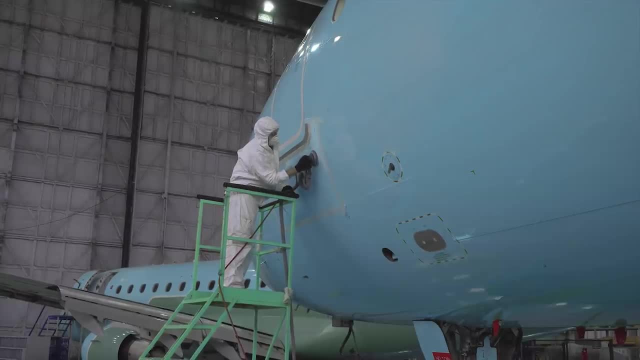 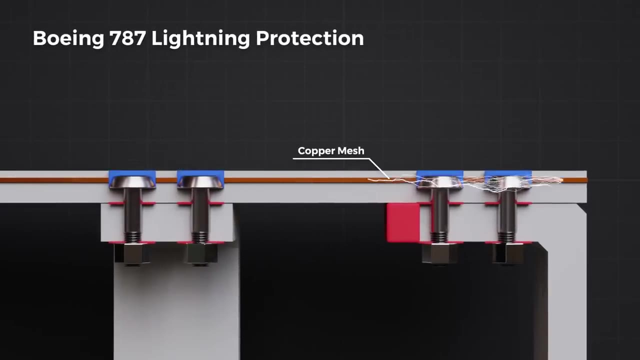 tests to ensure an accident like this could never happen again. Early 787 wings were designed with copper strips to ensure the electrons had a path of low resistance along the surface of the wing, ensuring they wouldn't travel to the fuel tank and cause a spark, while also preventing resistive heating damage to the composite. 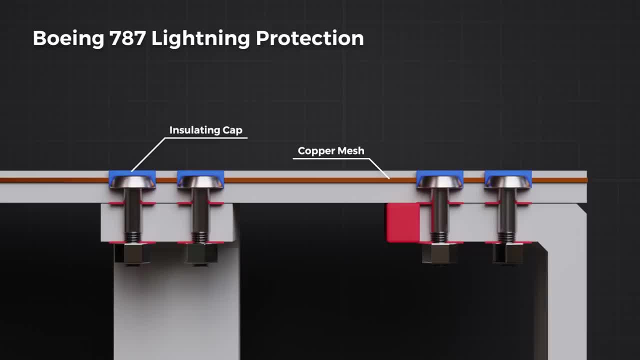 structure. Fasteners were sealed with an insulating material to stop electricity from travelling down the metallic fastener into the fuel tank. The engine of the fuel tank was only used in the early days of the airline, when it was fastener themselves were fitted with compression rings and a sealant to eliminate potential. 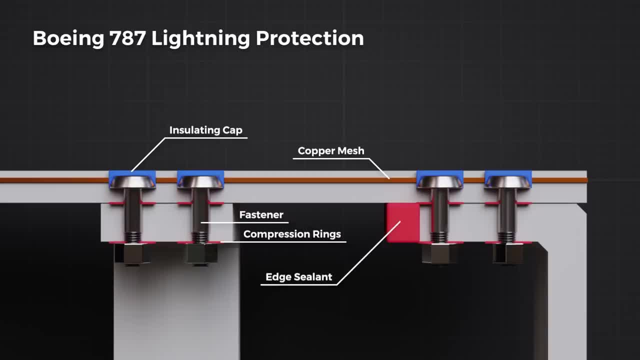 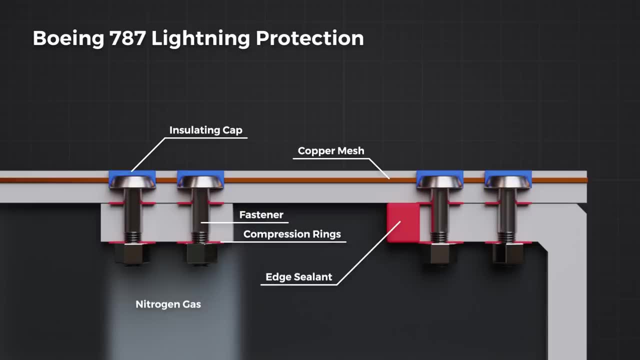 spark locations caused by gaps and sharp edges. Finally, the 787 has a nitrogen-inerting system that fills the tank with nitrogen. Ignition can't happen without oxygen. Boeing has since removed two of these protections in a cost saving measure, removing the copper. 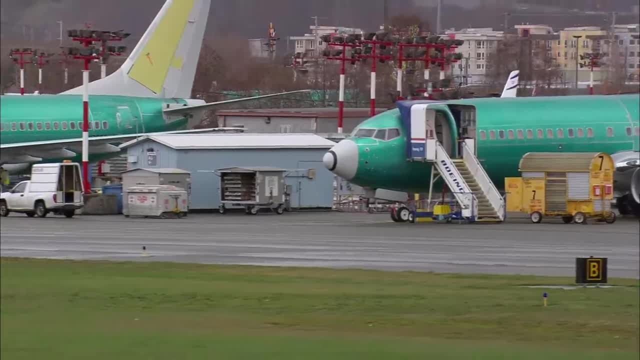 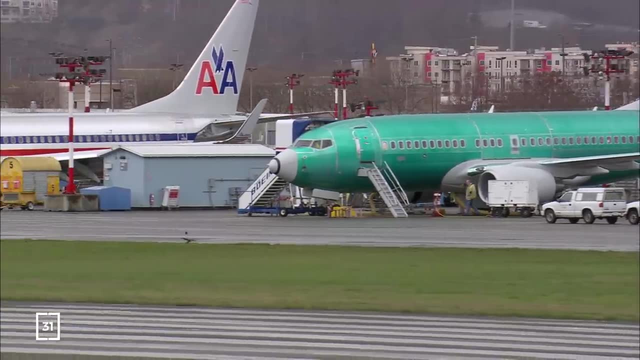 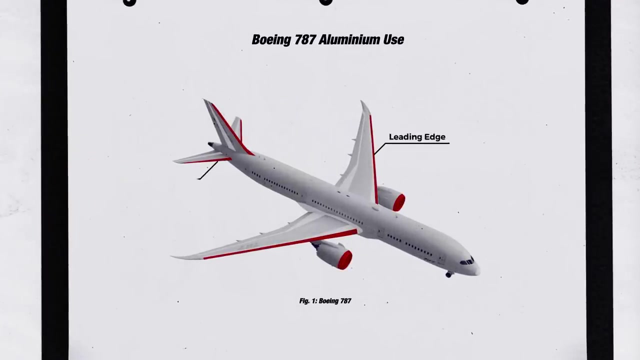 mesh and insulating caps, which drew concern and criticism, but Boeing argues that, between the nitrogen-inerting system and the other safety measures, these expensive features were not needed. Where composites couldn't be used, other materials were chosen: The leading edge of the wing and tail, the tail cone and parts of the engine cowling. 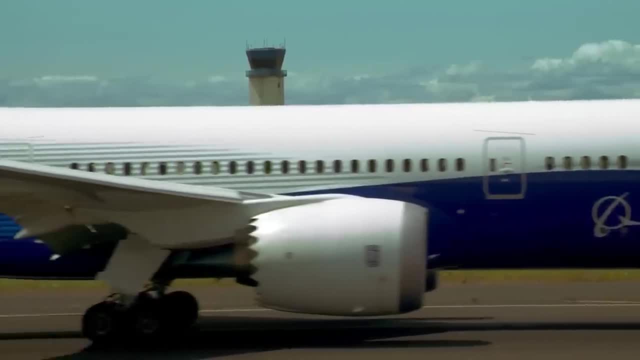 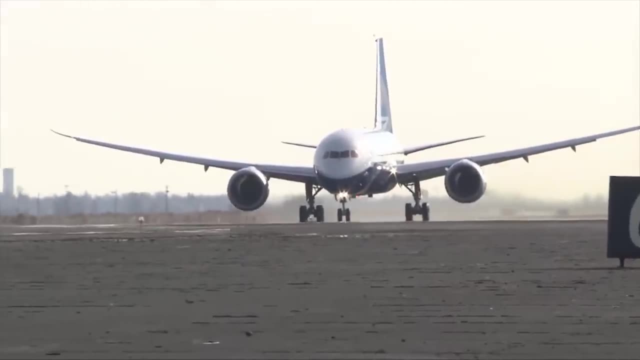 were all made from aluminium or other metals. The leading edges of the plane needed aluminium because of composites poor impact resistance. While composites have extremely high strength, they can be brittle on sudden impacts such as bird strikes, Which most commonly happens when the engine is not in good condition. 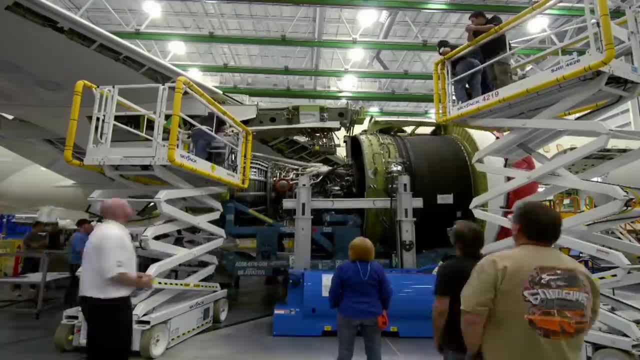 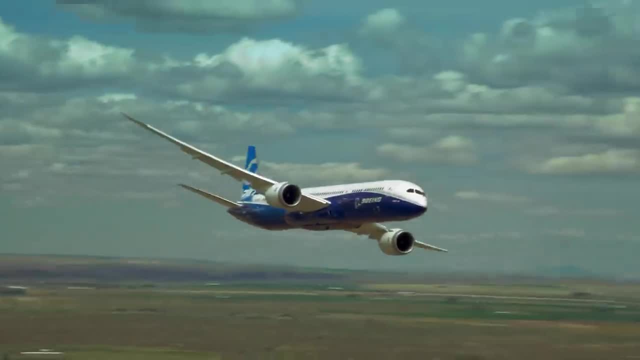 This may happen at the leading edge of the wing or on the engines. Metals are able to deform on impact with a reduced chance of fracture, instead of shattering as composites would. Aluminium leading edges were also beneficial for the purpose of de-icing, because it is 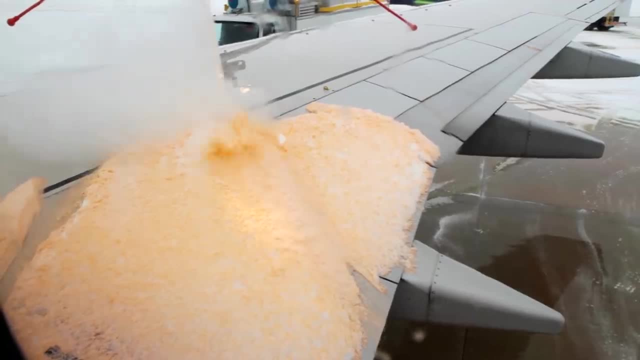 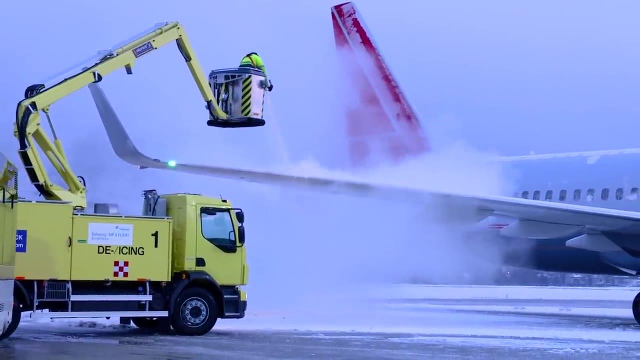 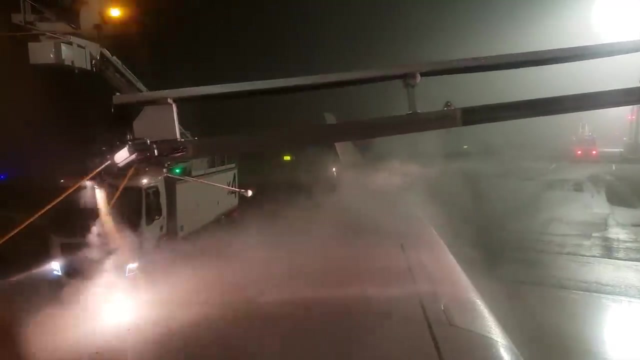 a good thermal conductor. If you have ever flown on a very cold day, you may have seen a truck spray fluid onto the wings of the plane. This is de-icing fluid, a heated mixture of glycol and water. It's needed because most planes aren't capable of de-icing themselves on the ground. 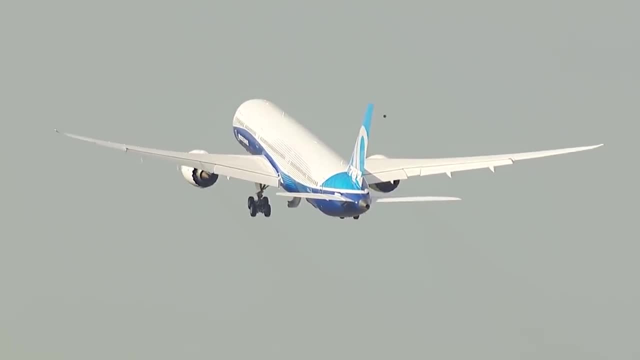 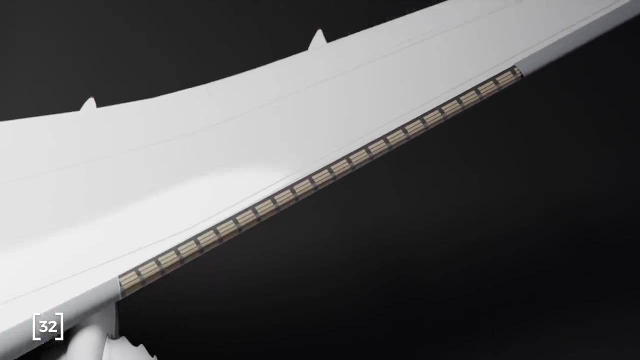 The 787 can when fed with external power, because it uses a new type of de-icing system. The 787 uses electrically heated blankets bonded to the surface of the slats, which are able to heat the surface of the wing and melt or prevent any ice formation on the leading. 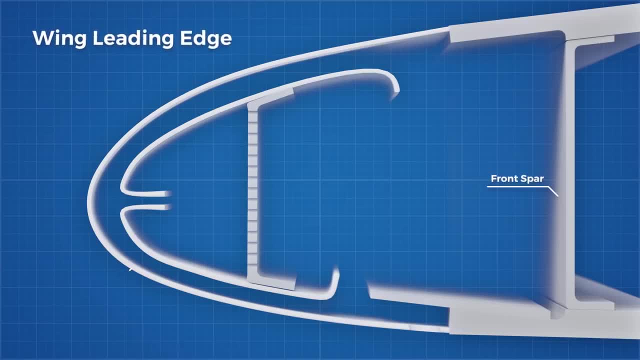 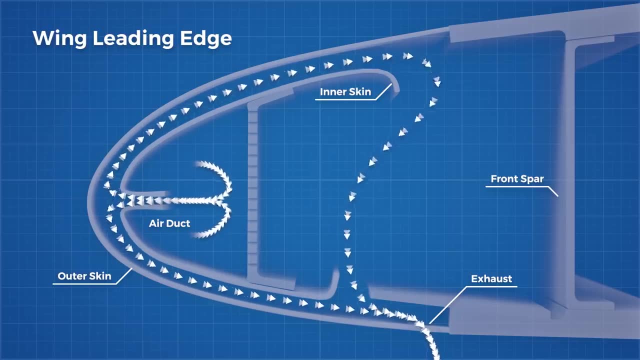 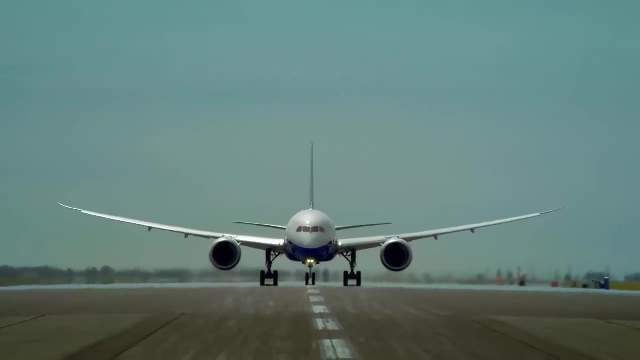 edge of the wing. Traditionally, ice is prevented by extracting hot bleed air from the engine and piping it to vulnerable areas such as the leading edge of the wing, where ice buildup could severely interfere with the wing's operation. This draws valuable energy away from the engines and increases fuel consumption, while also 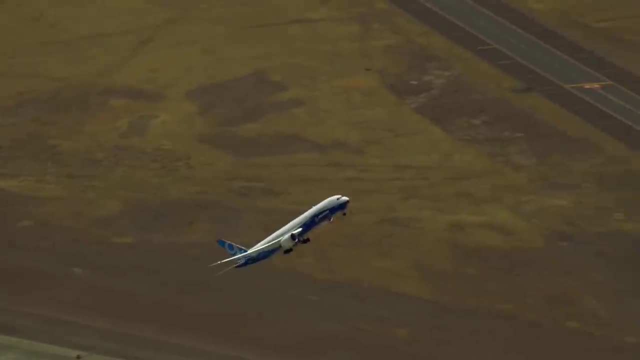 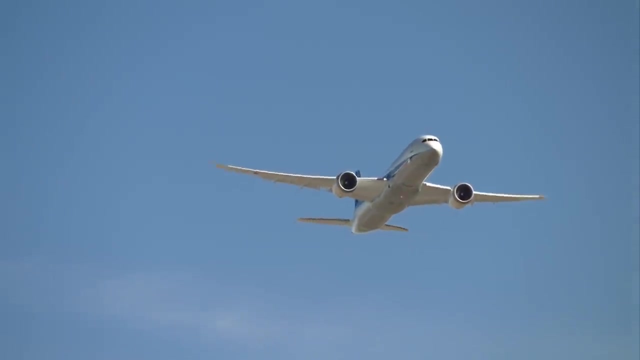 requiring a complicated network of tubing and exhausts, which add weight and increases complexity of construction and maintenance. The electric heating system is twice as efficient as the extracted bleed air system, as no excess energy is lost through venting air to the wing. Thanks for watching. 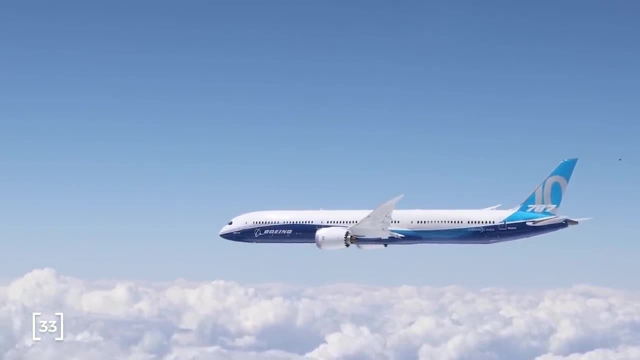 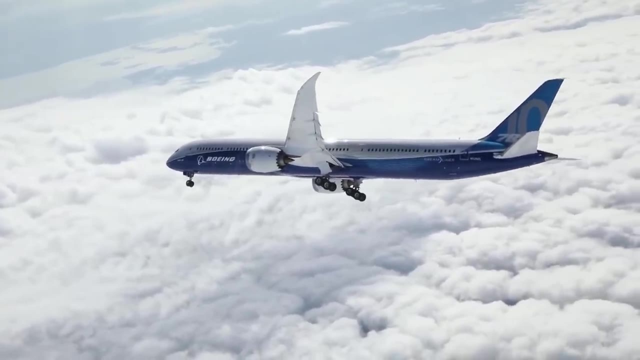 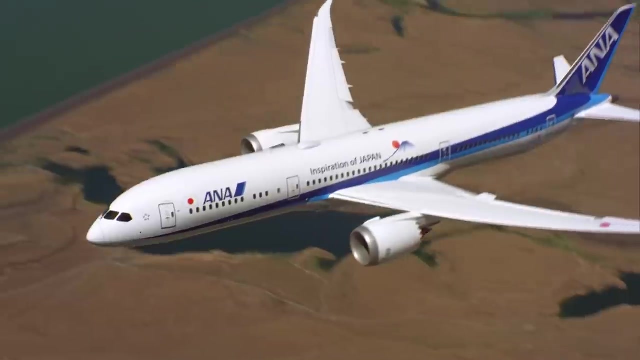 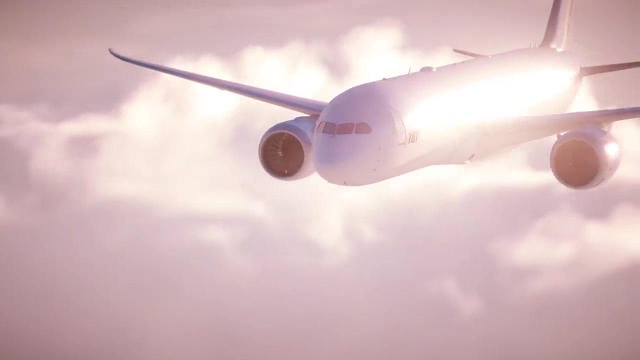 The 787 is actually the first commercial airliner that has eliminated this bleed air system, which was a huge technical challenge and required a complete redesign of several systems and an entirely new engine. In our next video, we are going to explore the incredible engineering behind the power. 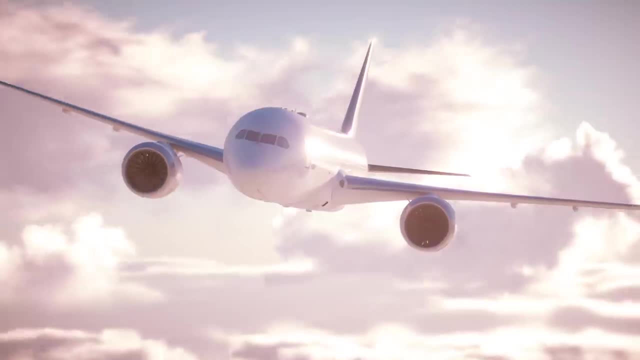 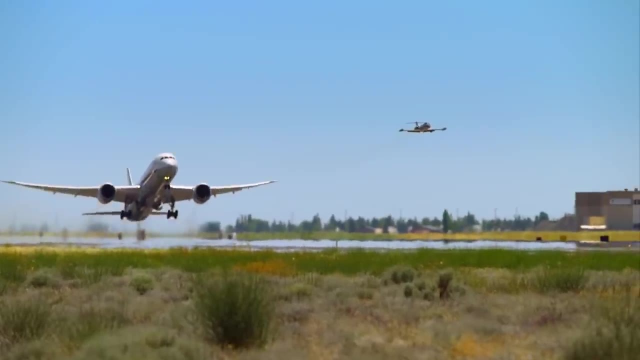 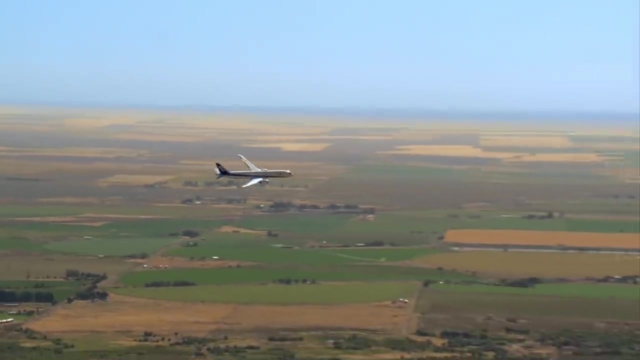 systems of the 787. Considering the advancements in the jet engine and the overall system architecture that allowed the 787 to become the most efficient long range airliner ever made, We will be releasing that video here on YouTube shortly, but if you don't want to wait, it's. 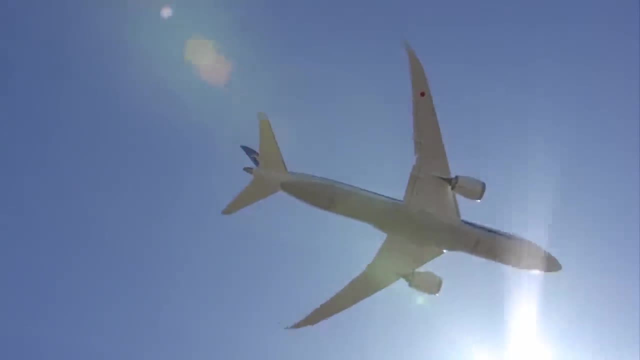 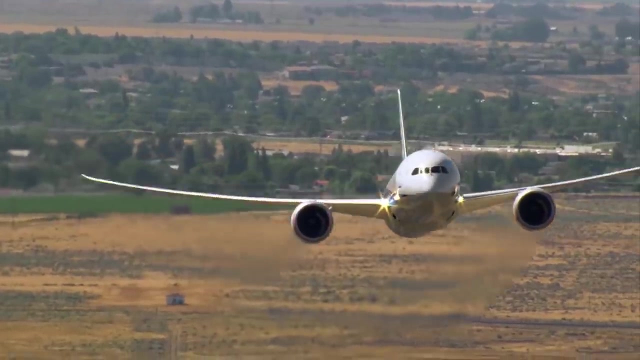 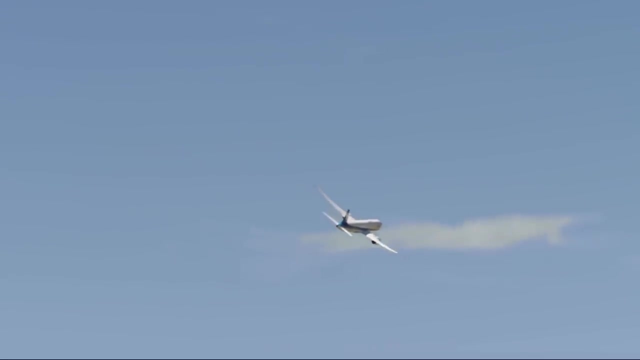 already on Nebula ad free. Or if you are like me and like to sit back and watch longer videos, We have created a special hour long version that combines both videos and has extra information that didn't fit into any of our videos. I have included links to both of these videos in the description, for those of you already. 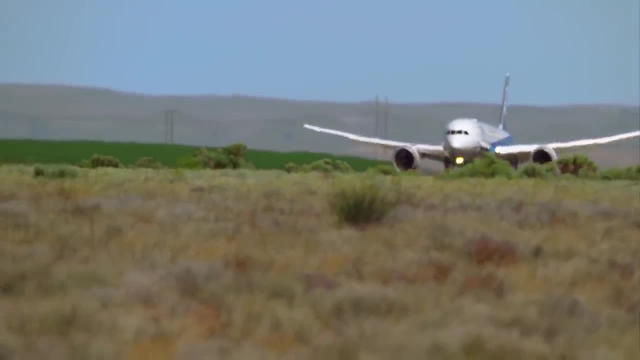 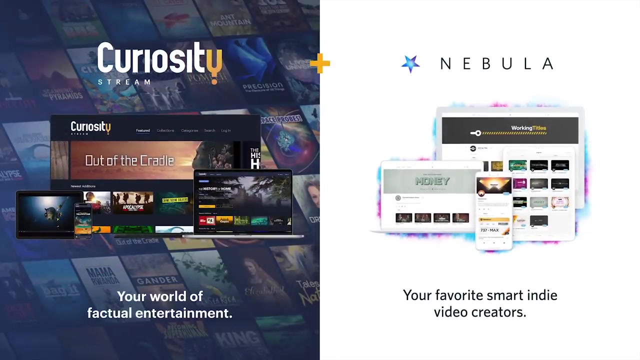 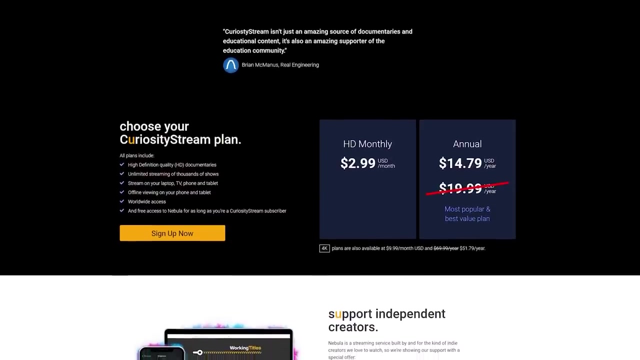 subscribed to Nebula Or if you have yet to start supporting the channel. there, you can sign up through the Nebula and CuriosityStream bundle deal for just £14.79 a year. That's just over one dollar a month, but that one dollar has a gigantic impact on this. 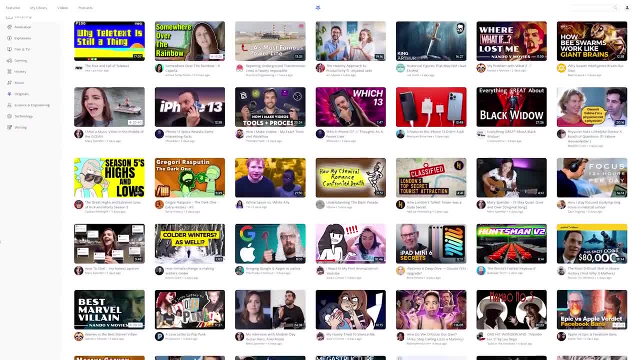 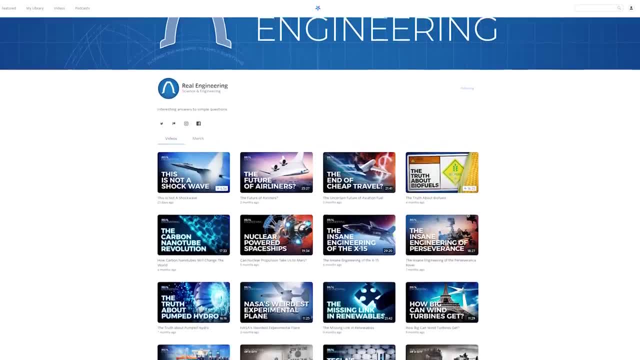 channel because we get to own and run our own streaming platform, And that gives us the freedom to create what we want how we want. If you are a fan of this channel, Nebula is the best place to watch everything we make. 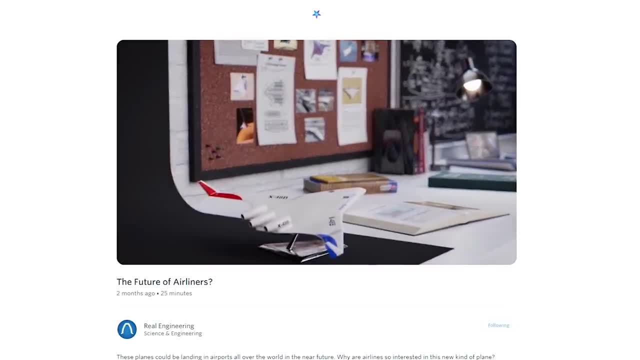 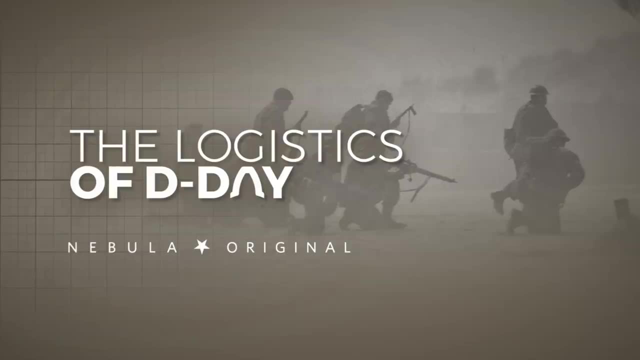 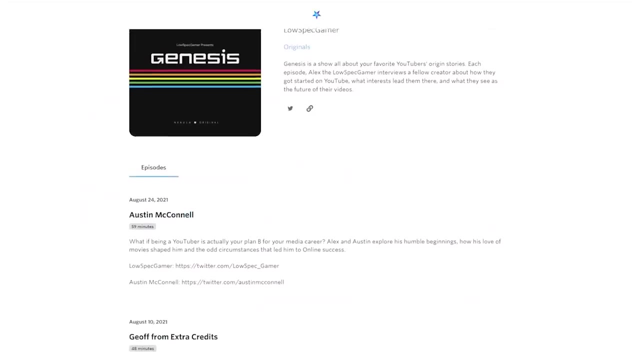 When possible, we upload our videos early to Nebula and all advertisements are cut from the Nebula versions of our videos. You can also get exclusive content from us, like our Logistics of D-Day series, or you could learn about my life before YouTube in LowSpecGamer's excellent Nebula exclusive. 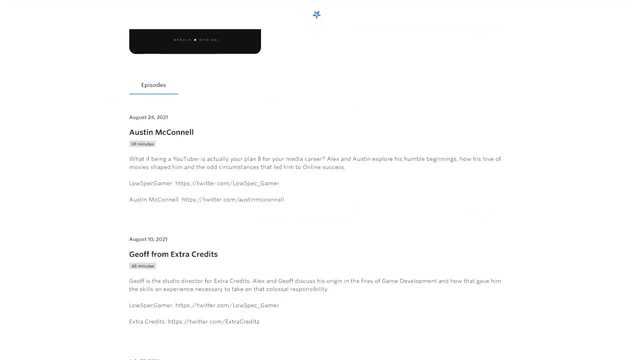 podcast Genesis, Where you can learn about my life before YouTube in LowSpecGamer's excellent Nebula exclusive podcast Genesis. Where you can learn about my life before YouTube in LowSpecGamer's excellent Nebula exclusive podcast Genesis, Where you can learn the story of how I quit my job in engineering to start this channel. 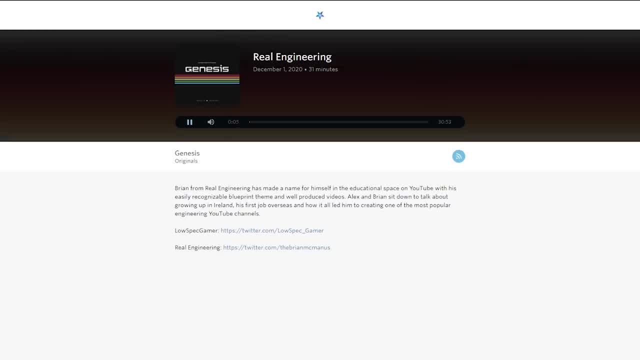 How advanced was the YouTube channel at that point that you were confident enough to quit your job? I don't think I'd uploaded anything at that stage. I can't remember. Wow, Wait, you quit before creating a YouTube channel- A little over one dollar a month. 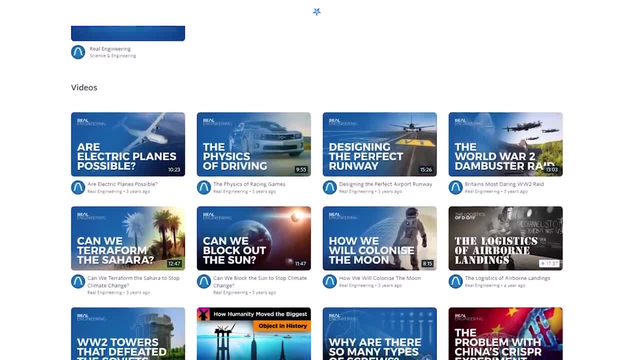 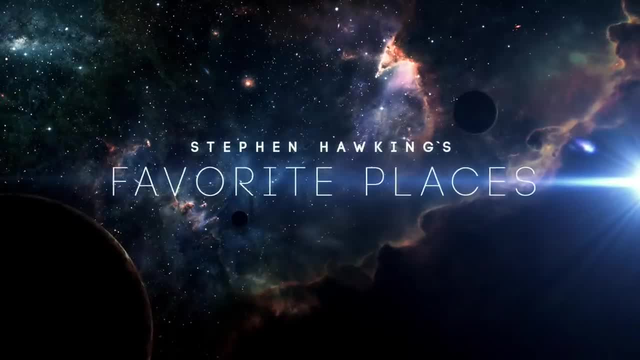 This is by far the best way to support this channel, and you get something in return, With access to both Nebula and all of the award winning documentaries on CuriosityStream, Like this fascinating biography on Neil Armstrong's life narrated by Harrison Ford. 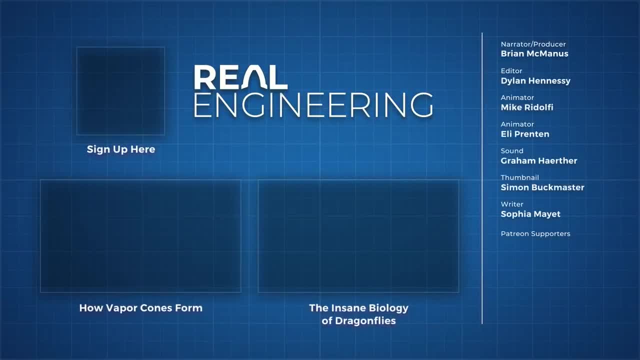 You can sign up to this amazing deal by clicking on this button on screen right now. or, if you are looking for something else to watch right now you could watch our last video on how vapor cones form on planes, or you could watch Real Science's video on the. insane biology of dragonflies.